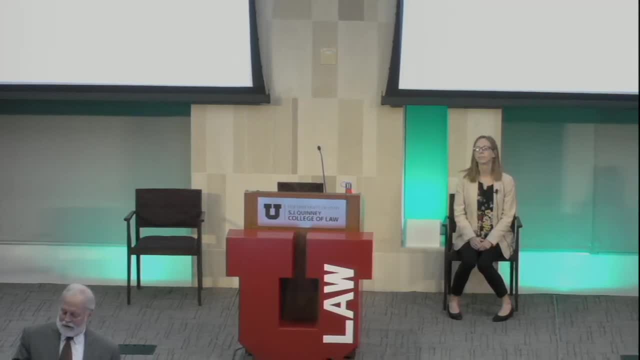 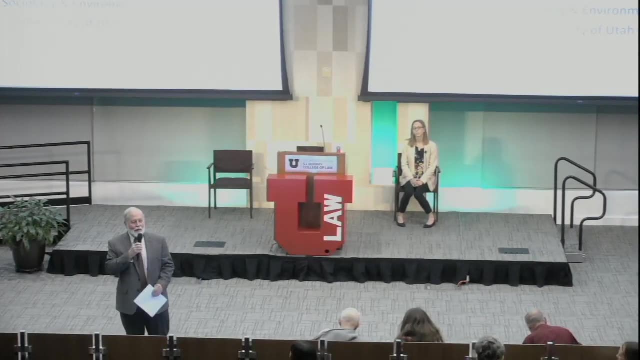 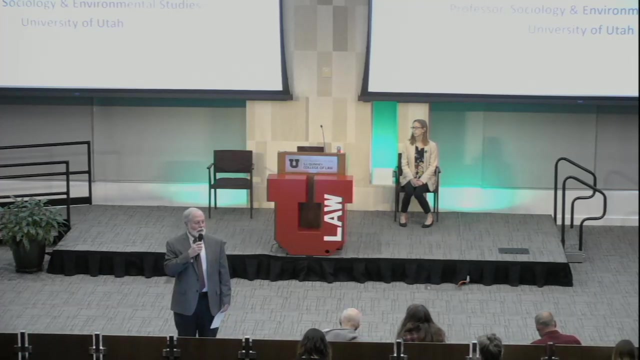 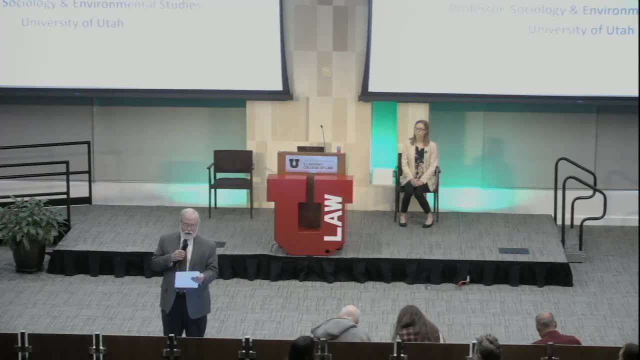 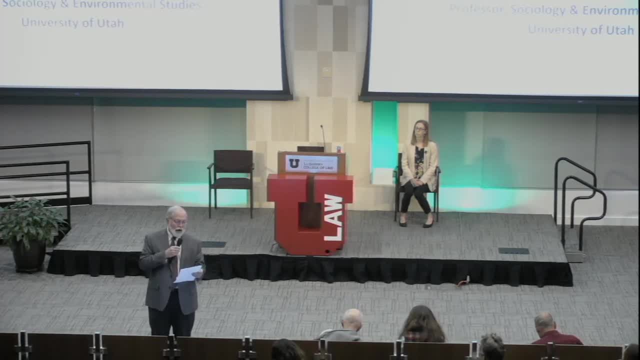 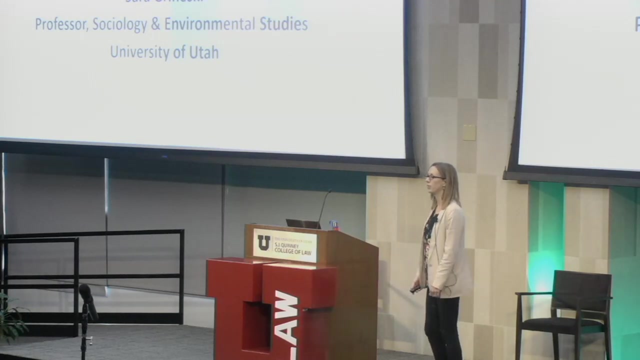 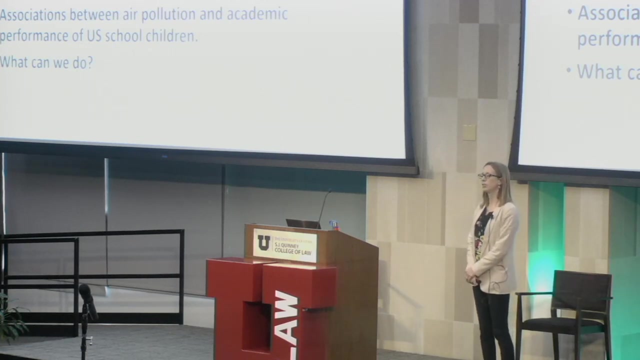 I'm Bob Kiter, Director of the Wallace Stegner Center for Resource Management. I'm Bob Kiter, Director of the Wallace Stegner Center for Resource Management. Then I'll go over the relationship between exposure to hazards and some neurological health effects. 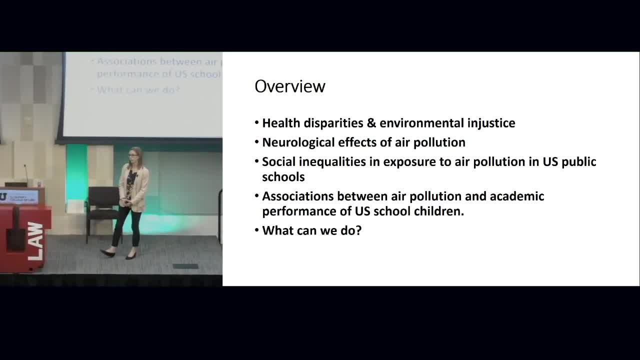 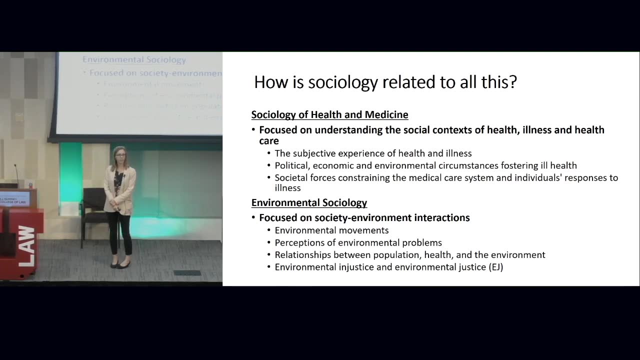 I'll talk a little bit about social inequalities and exposure, and also associations between exposure and academic performance, And then just a little bit about what we can do about all of this, because it is quite dire and clearly action needs to be taken. So, in terms of a general overview, I have a PhD in sociology. 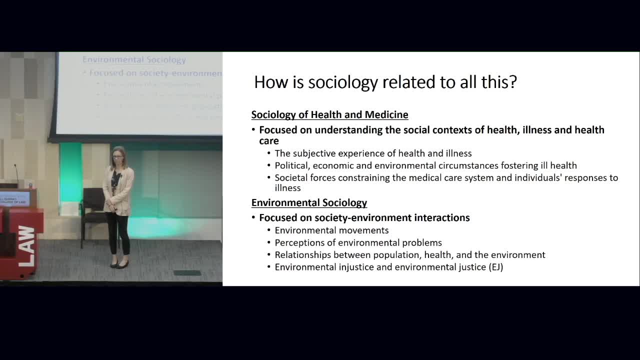 I'm talking about air pollution, in case that sounds funny to you- has sub-disciplines of Sociology of Health and Medicine as well as Environmental Sociology, and so my research brings together those two sub-fields, and you can see from my descriptions: medical sociologists sometimes focus on the political, economic and environmental circumstances. 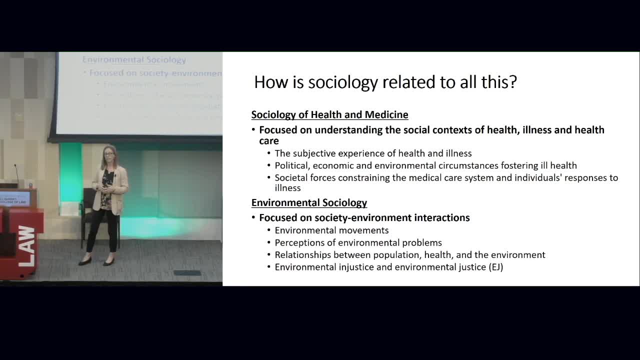 that lead to ill health, which is something that I connect with, and then in the environmental sociology realm, we're interested in relationships between health and the environment and also environmental justice, So that's how my discipline relates here to my work. So when we talk about 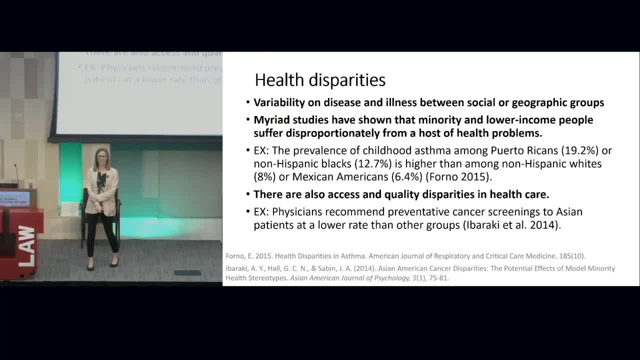 health disparities. we're talking about variability in disease and illness between social groups or between geographic areas. So, just as an example, childhood asthma, which is clearly a health condition that's closely connected to the environment. the rates of asthma vary quite dramatically between different racial ethnic groups. Puerto Ricans, for example, in 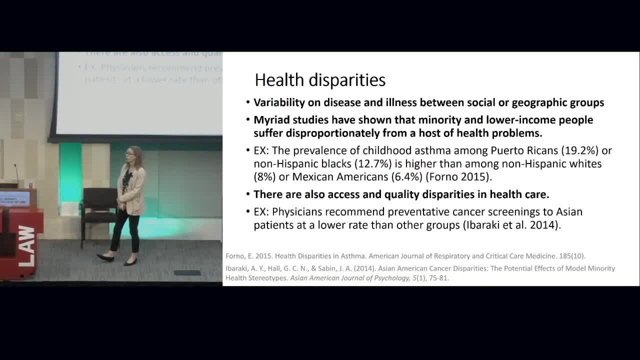 the United States have the highest rates of asthma, whereas Mexican Americans have the lowest rates of asthma. So that's an example of a health disparity, a social inequality in health or illness. There's also disparities that sociologists study in access to healthcare and also in the quality of healthcare received. And then on the environmental side, the area. 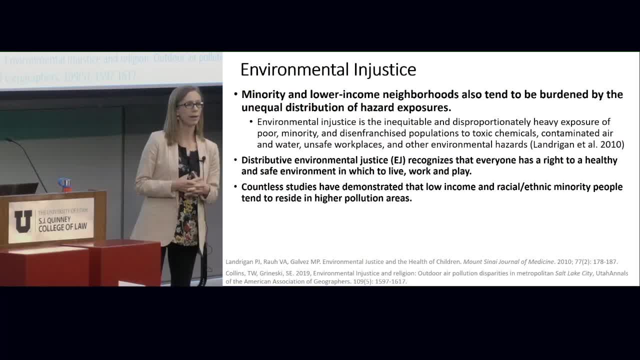 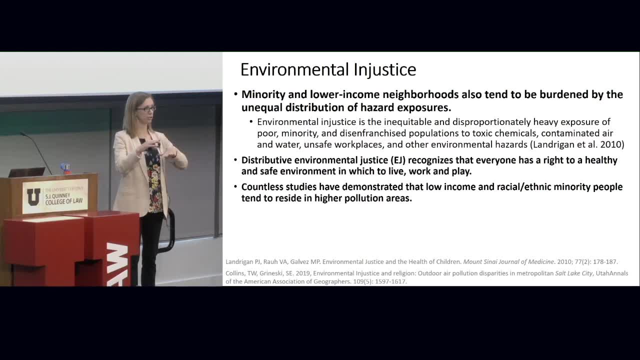 of environmental injustice. when I say environmental injustice, what I'm talking about specifically are distributional environmental injustices, which has to do with the distribution of humans and hazards in space. So there's many, many studies that show that people of racial, ethnic minority backgrounds and people 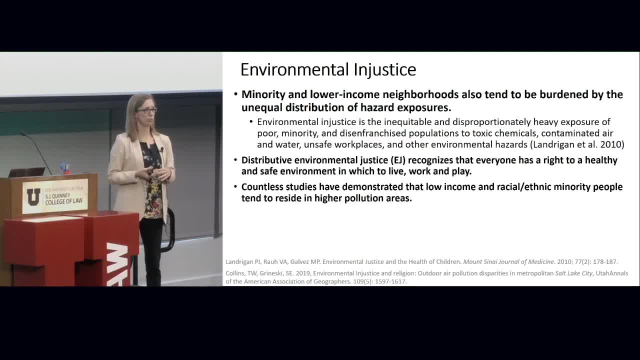 of low income tend to be burdened unequally by the distribution of hazards. So one thing to note is that we clearly see this here in Salt Lake City. So we recently did a study looking at patterns of distributional environmental injustice in Salt Lake and I will say, as someone 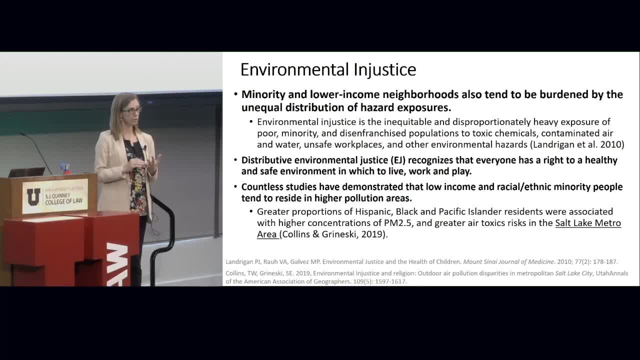 who's done this type of research in Phoenix, Houston, Miami, Ciudad Juarez, Mexico, Tijuana, Mexico and El Paso. we had the strongest relationships here in Salt Lake City of those places that I've studied- Very strong patterns between Hispanic, black and Pacific Islander. 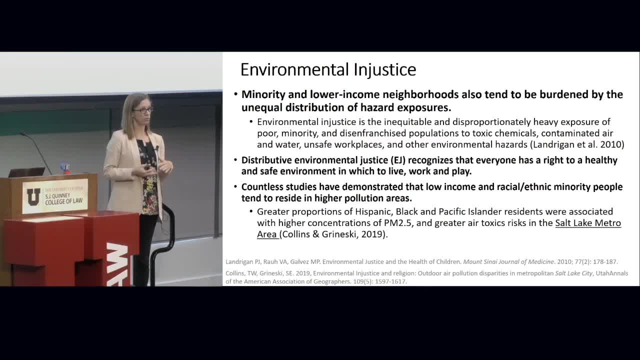 the composition of those groups and neighborhoods, and then a variety of air pollutants, including PM2.5 and air toxics. So we clearly have these patterns here. I keep forgetting. I have a clicker. I don't usually teach with one of these. 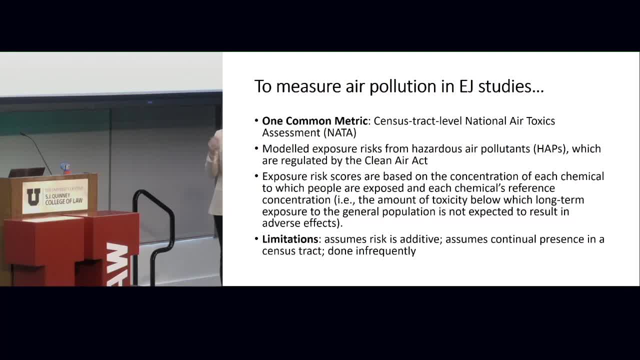 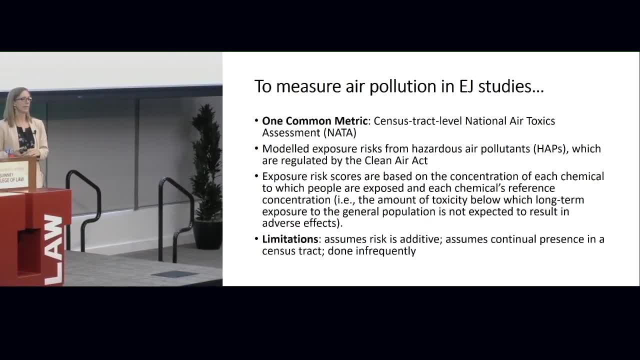 All right, So I just want to start briefly by introducing you to a data source that I'm going to use throughout the talk today as I talk about my own work. So one source of air pollution data that people use when they're studying patterns of environmental injustice is what's. 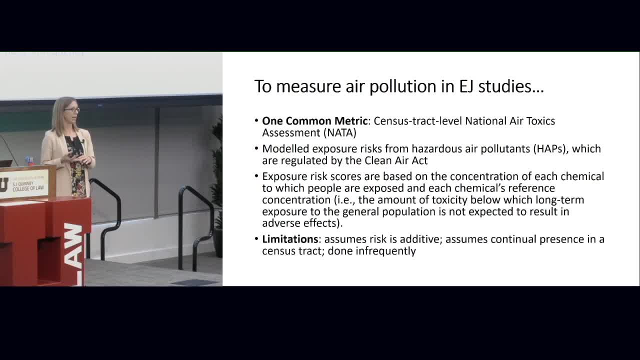 called the National Air Toxics Assessment or the NATA. This is a census tract level measure so you can make a map of the entire United States shaded by the level of air toxics exposure. The NATA is a product of the EPA. They basically do really fancy modeling and they also weight their models. 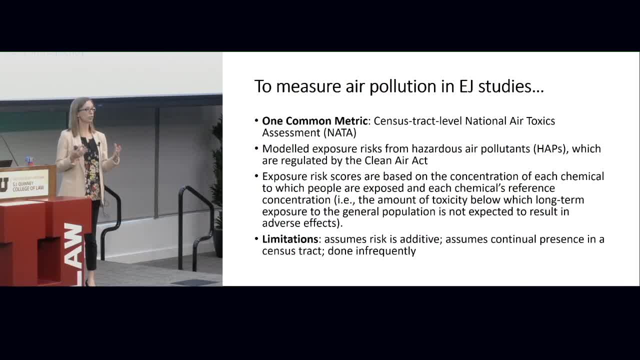 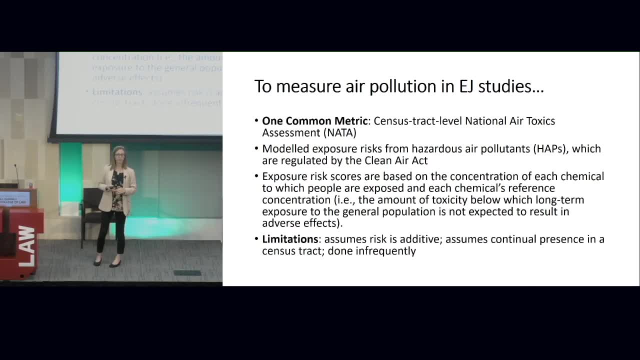 by health risk. So, for example, they have like a cancer risk score, which is one that I'm going to use, and it means higher levels are higher levels of cancer causing hazardous air pollutants being released in those census tracts. So this is a great source of data because it's spatially. 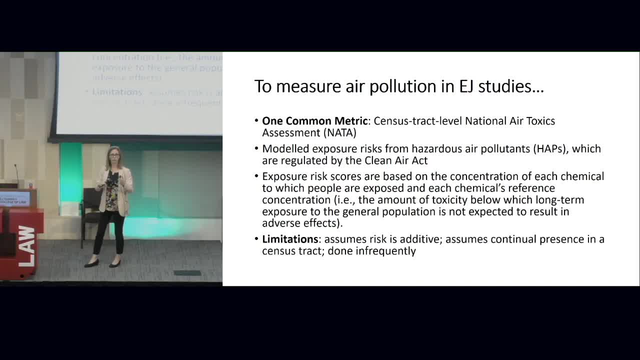 quite useful in neighborhoods. We often think of census tracts as neighborhoods. They're not all that large right, which is good for this type of analysis. There are some limitations. They don't come out with this every year. It's very intensive. 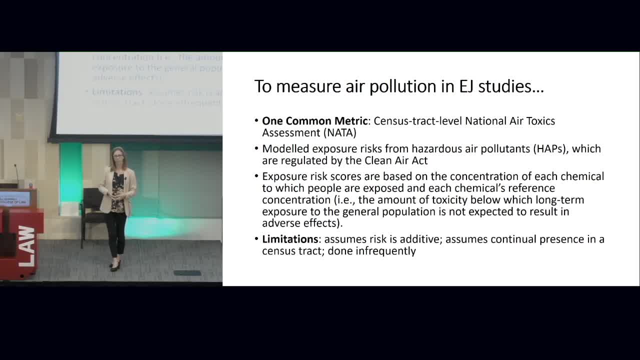 So, like the most recent ones are 2011 and 2014.. So there are limitations with this measure, but it is a very useful measure for the type of research that I do, and so you'll see this measure today as I present. Here's one example. So this is a national level study that we did, and this graph 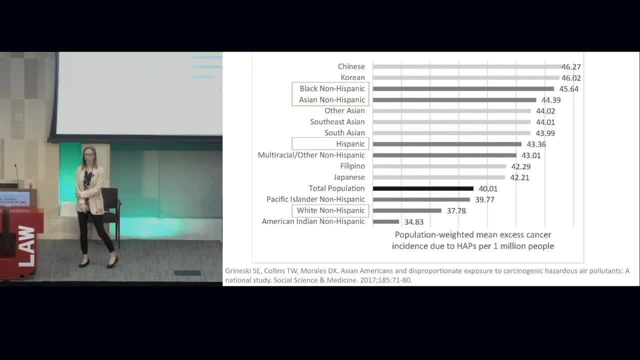 just uses that NATA, specifically the cancer risk, and the actual measure is excess cases of cancer due to exposure, to hazards and to risk. So this is a whole other level of data And it's very as air pollutants above and beyond what you would already expect in a population. 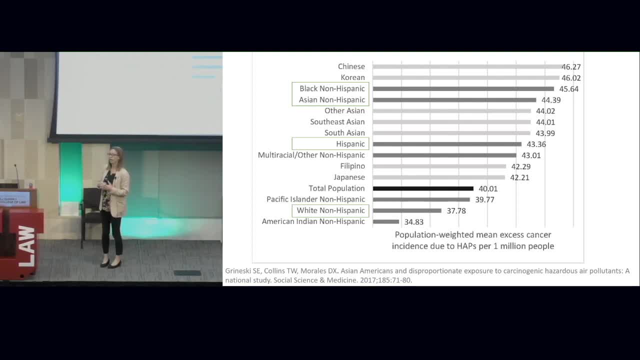 So you can see that in terms of patterns of inequality, right, you see black and Asian Americans having high risk, Hispanic having a little bit lower but well above the risk of white and the total population. This paper focuses on Asian American groups, hence the other groups in there, and it's 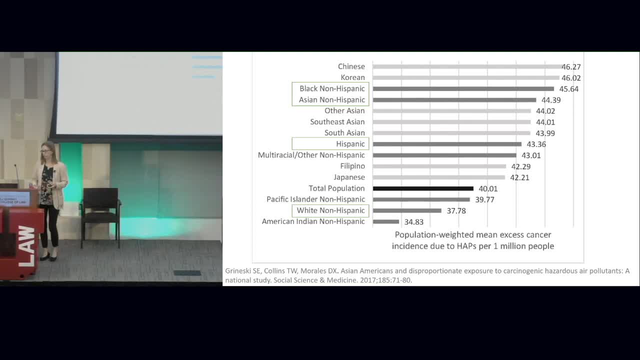 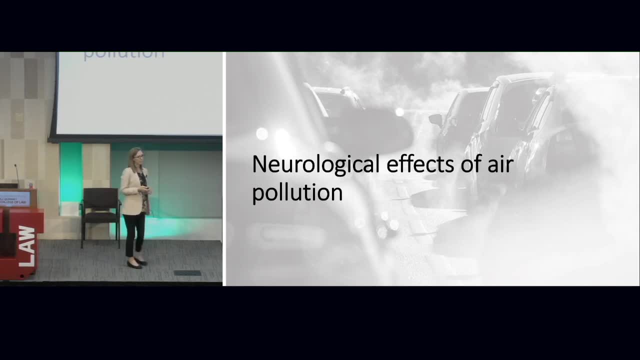 worth noting that Chinese Americans have very high exposure to residential air toxics, So that's just an example of how the NATA looks. So the next thing I'm going to talk about today, as related to my focus on children's academic performance, are the neurological effects of air pollution. 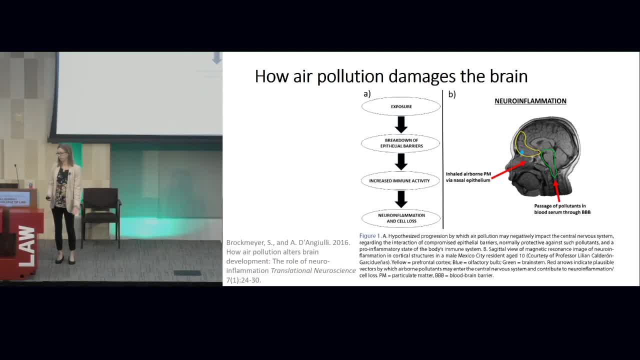 I don't know about all of you, but when I started doing my own research on air pollution, I was focused on asthma. right, I think air pollution, I think respiratory effects. Then I learned actually there's cardiovascular effects of air pollution. and now in the last, 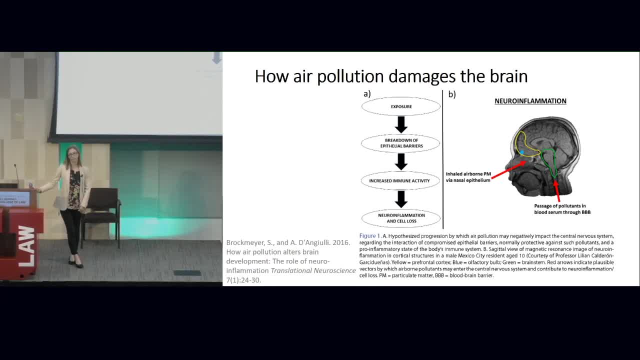 five years I've been learning about the neurological effects. So what are the neurological effects of air pollution? This is an area of research that was very, very small 10 years ago, even five years ago, and now, every time I try to write an article, every month, I have to update my literature. 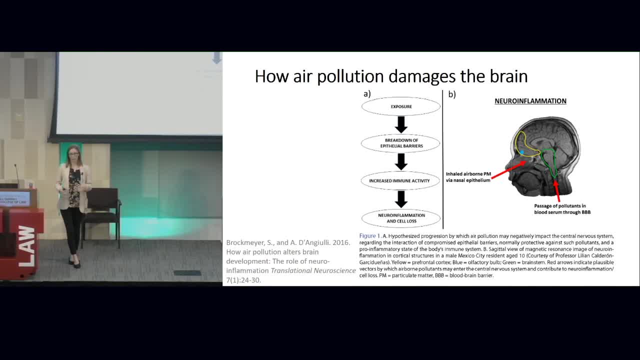 review because new research is coming out all the time now in this area. It's a very important area of research. So how does air pollution damage the brain? I took this graphic from a lit review and basically it talks about exposure to air pollution. 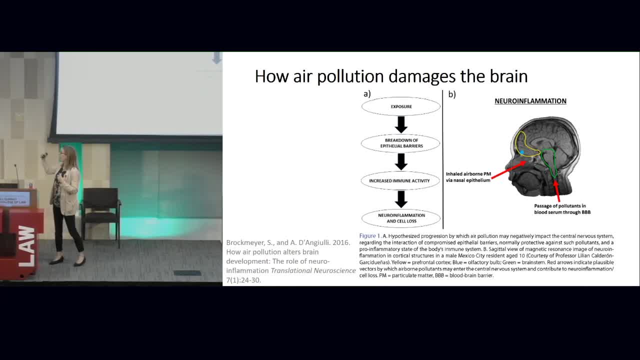 how does it affect your immune system? how does it affect your immune system? And so it really goes down the epithelial barriers in our bodies- right. And then our body tries to fight off these invading air pollution cells- right, and we increase our immune activity. 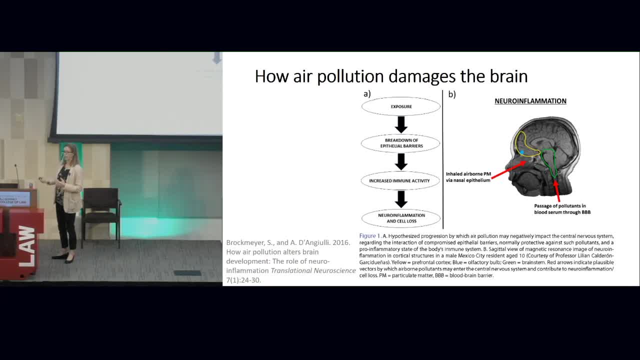 We have this big immune response and it causes neuro inflammation and cell loss in our body. This happens in our brain. There's a professor at the University of Montana, Lillian Calderon, and she does research in Mexico City and she does autopsies on otherwise healthy people who die in traffic accidents. 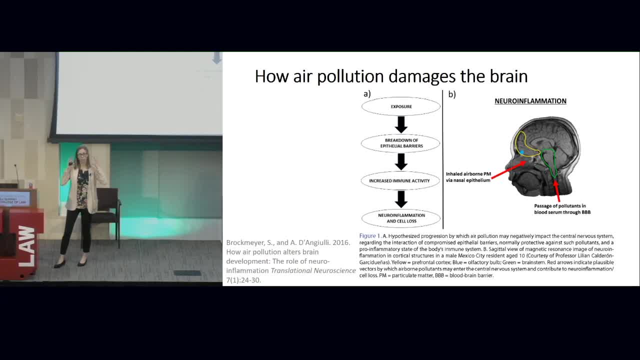 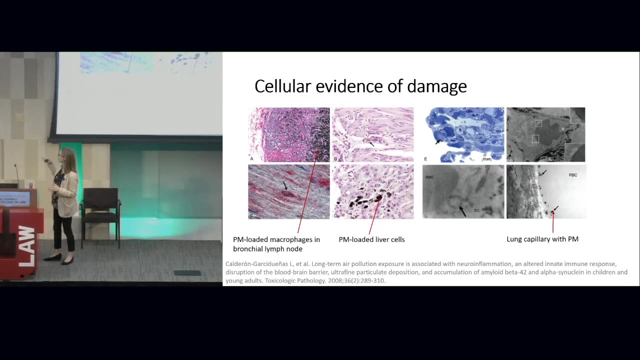 seen in young teenagers structures in the brain that look like they have early onset Alzheimer's disease. so there are clear physical damages that happen in our brains as the result of exposure to air pollution. here is some slides from one of her articles. I didn't label them all for you, but you can see at a. 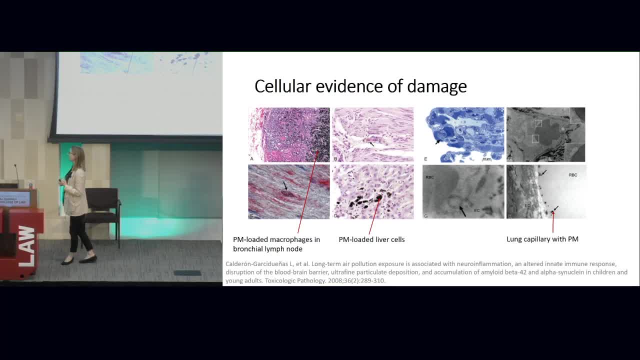 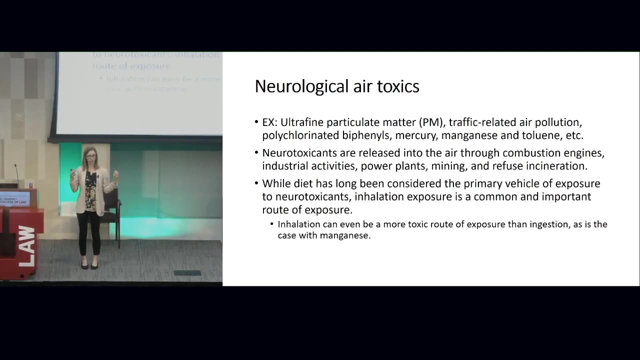 cellular level that our body, right, we take in the air pollution, it crosses the blood-brain barrier and then it's found inside our body and our body tries to fight this off. so when I talk about neurological air toxics, you can think about in general how air pollution causes this neuroinflammatory response. 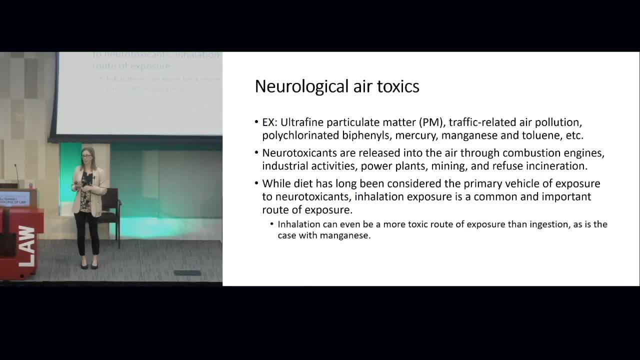 and causes damage. you can also think about specific toxics that are known to be damaging to the neurological system. lead, for example, is probably the one that most people are most familiar with. so previously, when people were thinking about neurotoxicants, they tend to think about how we ingest them, right, you think? 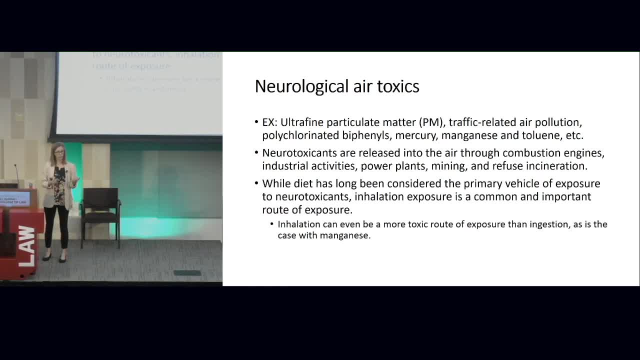 about little kids crawling on the floor of old houses eating paint chips, which is a key way in which we do ingest neurotoxins. But we also ingest, we also breathe them in. We inhale them as they are released by power plants, mining activities, combustion engines, etc. And there's some. 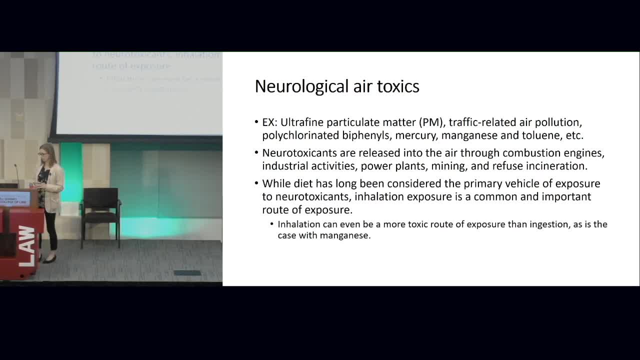 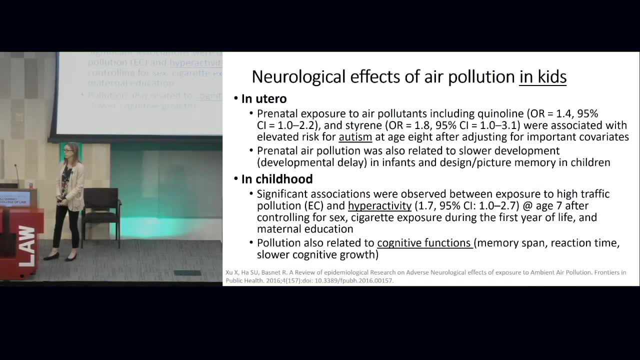 emerging evidence that this inhalation pathway might even be more dangerous than an ingestion pathway. But no matter what, you don't really want to be putting these things in your stomach or your lungs. So, in terms of the literature, there are many literature reviews that have come. 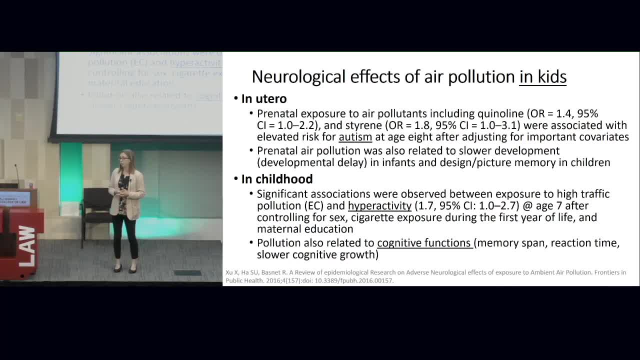 out in recent years, highlighting all the different ways in which air pollution affects children, adults and older adults. So, for example, prenatal exposure to air pollution has been linked to autism and ADHD more generally, slower development, developmental delays right, And it's also been 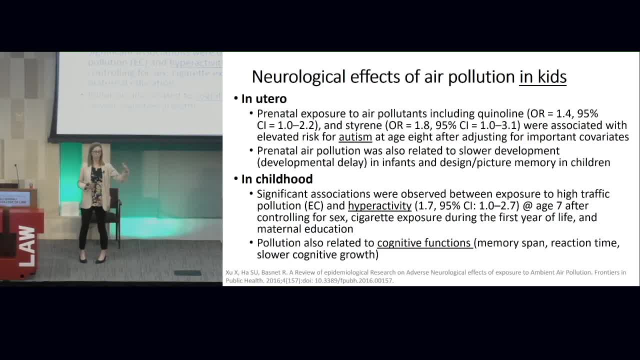 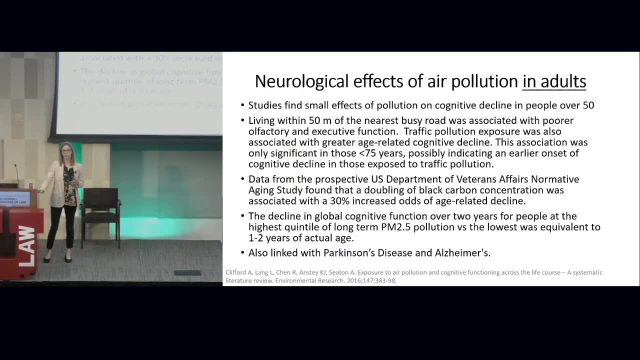 associated with cognitive functioning of children And they look at both exposure in utero and infants And they look at both exposure in pregnancy, in childhood right, And different studies use different metrics, But the general trend is this: association. There are also similar associations in adults and specifically in older adults. This important 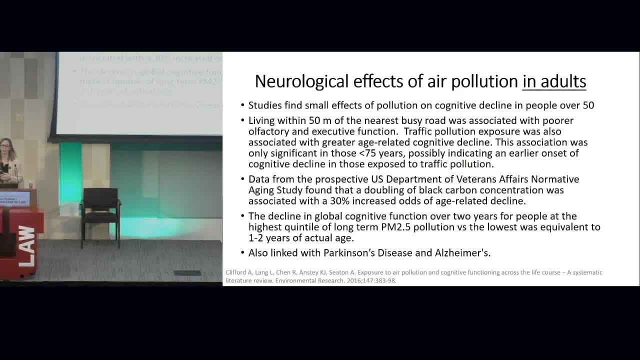 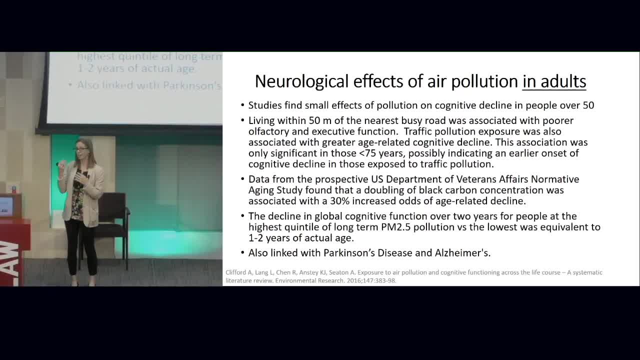 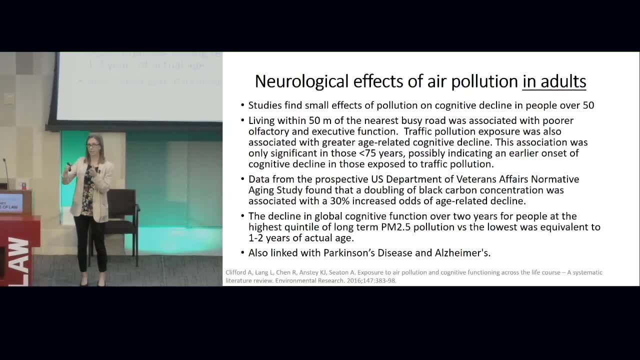 age. So there's other type of also been linked with Parkinson's disease, Alzheimer's disease, et cetera. So that's a brief overview on the neurological effects of air pollution. For me and my own research that's quickly crippen, That was essential. But it's a big conversation ahead. What is becoming our new sort of first goal and our new goal? Peace of mind, ularising the world before we know it? Well, given how the worldwide news and the public isn't interested in making a such fontic. 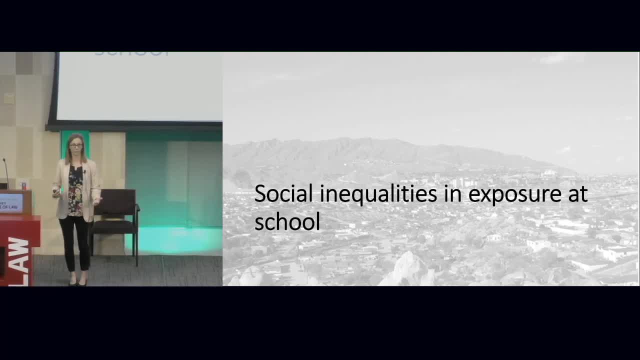 attacks like this. it must not be worth doing it. It sufficient to have a lot of choice. positive thinking about the responses to the media"沒有 100%. that's far beyond the scope of what I do. right, I don't do autopsies, thank goodness right, but I 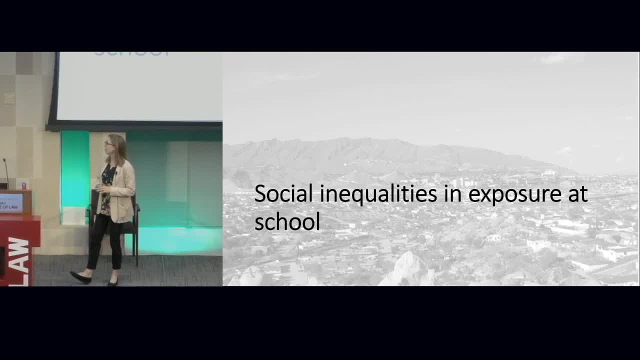 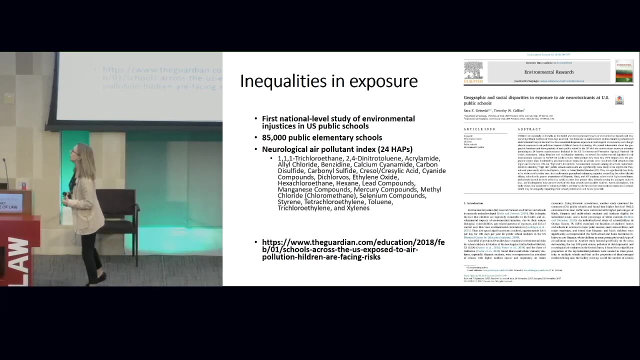 study the social side of things as a sociologist, so one of the things that I'm interested in is this situation of distributional environmental injustice and social inequalities and exposure. so we did a study, which was, I guess, a year ago now 2018, published in 2018, and we looked at 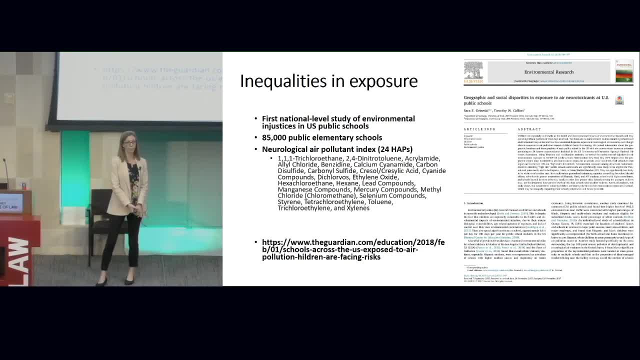 the locations of all the public elementary schools in the United States. there's a great data source from the National Center for Educational Statistics. you can get data on public schools any year, any state right. so we downloaded all the data. I downloaded all the data for the 85,000 roughly public schools in the United States. I picked the year 2011 because 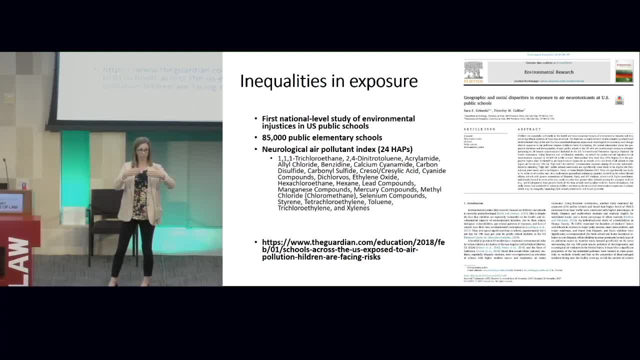 if you remember the NATA data from 2011, it matched that up. the 2014 NATA wasn't released until after this study was published. so, and because I have this interest in the neurological effects of air pollution, I created an index based on the level. 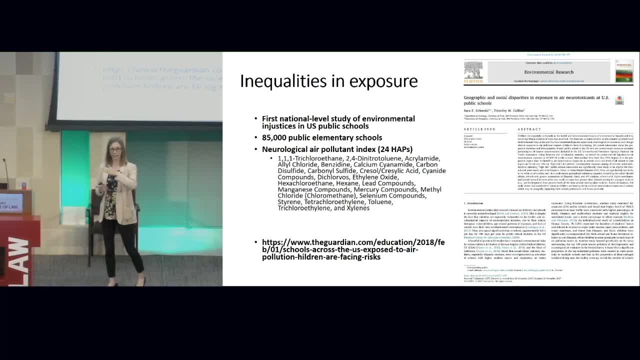 of neurological air toxins in the neighborhood or the census tract surrounding the schools. so included in the NATA are 24 unknown neurotoxicants based on EPA, a listing of these things. they're all there long fancy names, except for some like lead right, which is not quite so fancy. 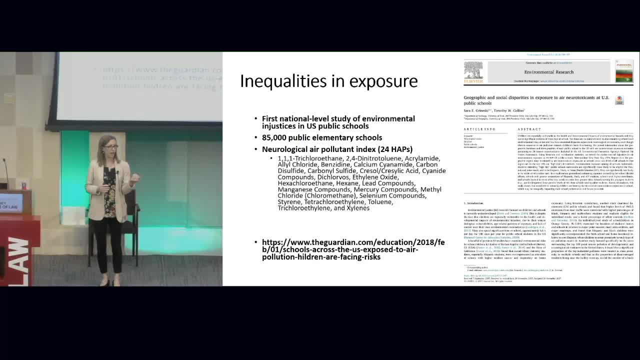 but this is good. so I created an index and then we looked at the sociodemographics of schools as related to exposure to neurotoxicants. based on this index, I was surprised this study got more attention than anything else I've done previously, and I don't know if it was that much more exciting. 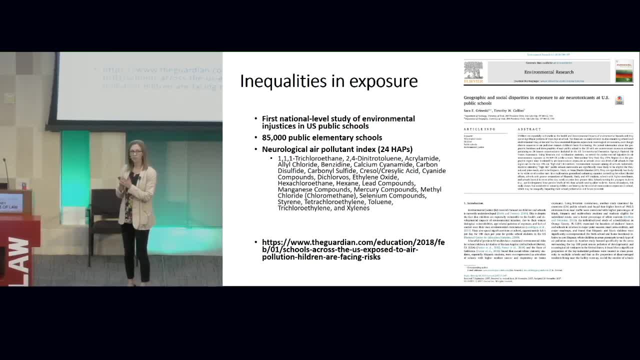 or better, done right. who knows how these things happen, but the Guardian, for example, did a pretty long story. my article is much less interesting than the Guardian, which is why I put that link up there, for you went and talked to people in New Jersey that lived in these areas of really high 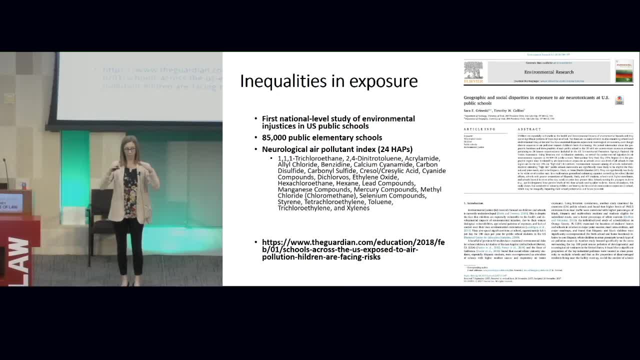 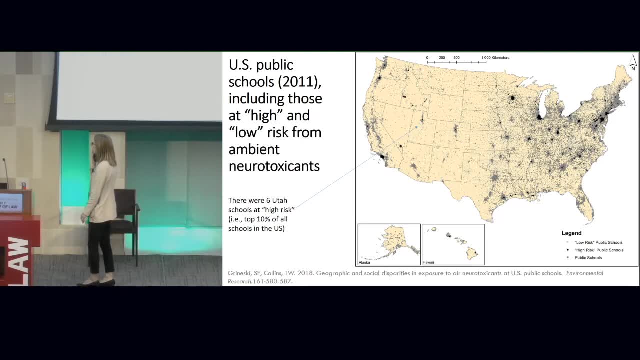 risk and did a really nice story that fleshes out the picture much more than our paper does. So what do we find? Well, here's a map of all the public schools in the United States. because of the requirements to publish in grayscale, you should have this one, like red and green, right, but the dark black dots are the 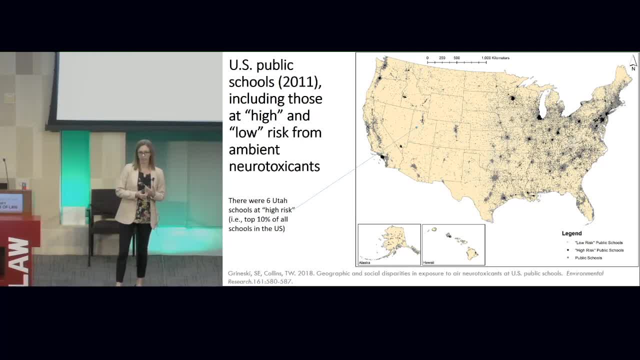 schools that are in the top 10% of all schools in the United States for risk based on my index of ambient neurotoxics. So of interest to you might be that there were six Utah schools that fell in this top 10.. So we have. we have about. 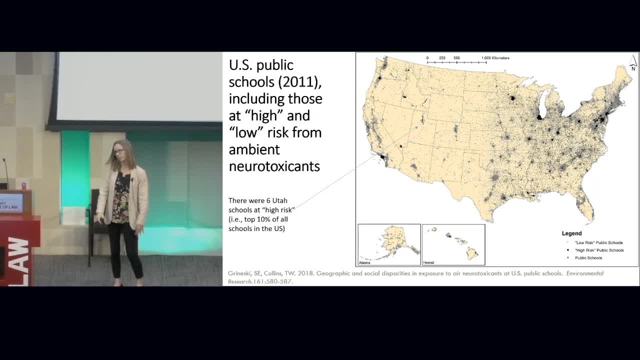 8,000 schools in the top 10%. right, because we got 80,000 schools. but there are six Utah schools that fell in that that top group. Five of them were in the Granite School District and one of them was in the Salt Lake Independent School. 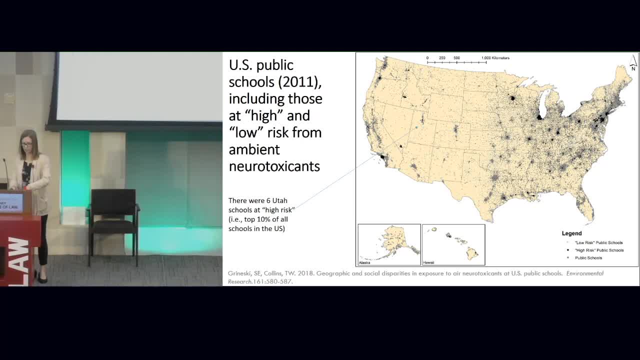 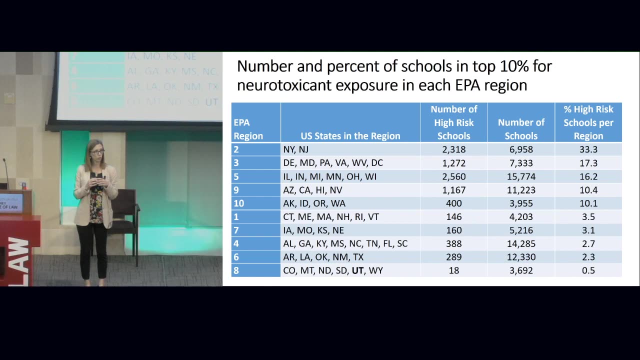 District. So while you're in the Granite School District, you're in the Salt Lake Independent School District, And while Utah isn't dramatically affected, we do have some specific schools that are located in areas where there are a lot of of ambient neurotoxicants. So what we did in the paper then was we looked at the 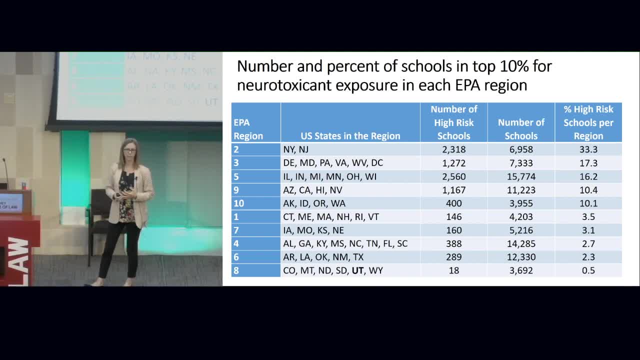 proportion of schools at high risk right in this top 10% in the different EPA regions, since quantifying things by EPA region is somewhat useful since EPA regions make decisions and are in charge in, in some degree, of the environment in that region. So Utah is not the most. 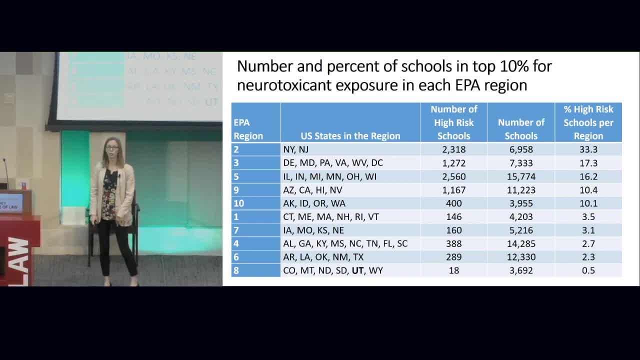 how you can see, we're at the bottom right Sort of the Mountain West- is lower in terms of social inequality and exposure to these hazards. The top EPA Region 2,, which is basically New York City, had 33% of all the schools in those two states are located in the top 10% of the most hazardous. 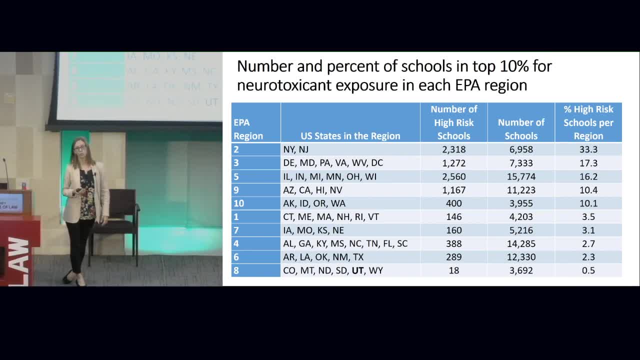 schools in the country for this ambient neurotoxicant measure. So it's a serious issue in New Jersey and New York and I think that's why the Guardian article focused specifically on that region, because it's a pretty serious disparity there geographically. Then we can. 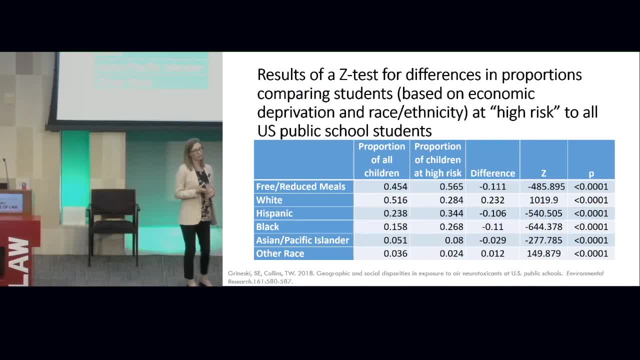 also look at the data at a national level and compare the demographics of students attending high-risk schools to the demographics of all the students in the United States, And that's what this basically does. So let's look at the percent at the white row. So in the United States at all, 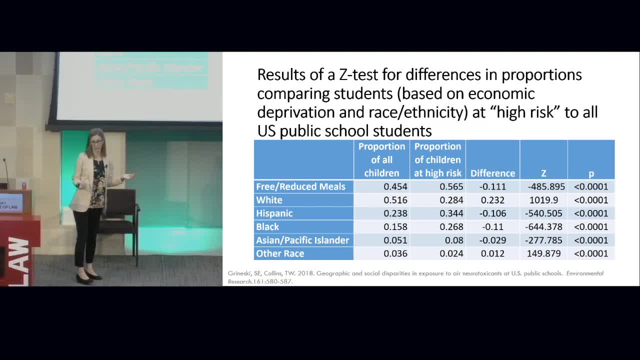 of our public schools, 52% of all the kids are white. 52% of US public school students are white or they were in 2011.. And then you can see that 28%, right 0.28, is the proportion. 28% of all children at the high-risk schools are. 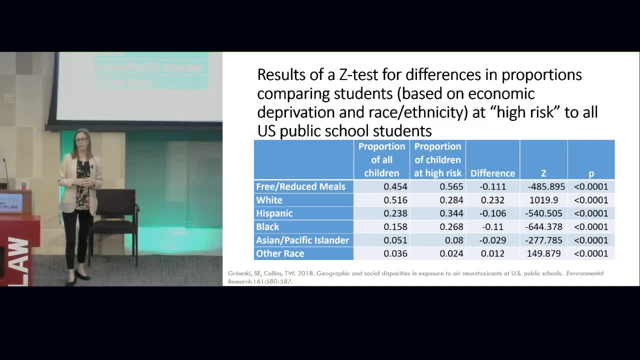 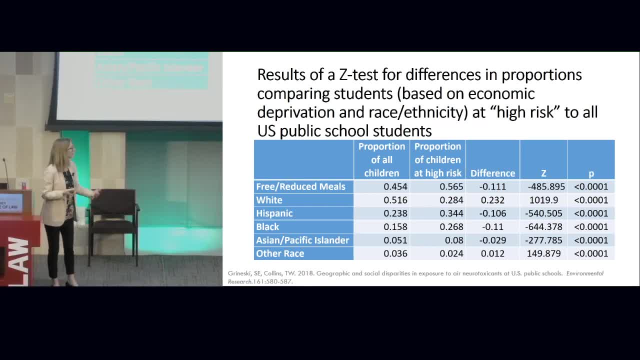 Black and Asian and Pacific Islander children are over-represented at schools at high risk right. So Black children make up about 16% of the public school population in the United States and 27% of the population in the high-risk schools. So you see this racial disparity in students attending. 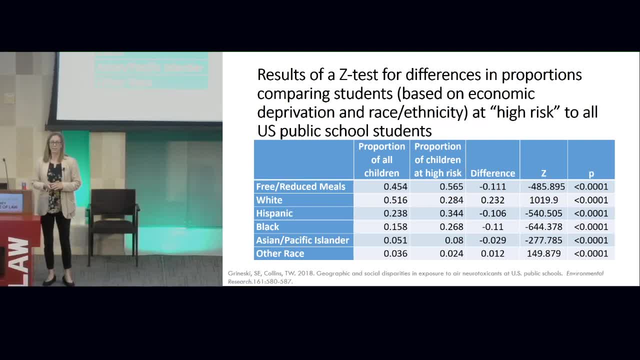 these schools that are located in high-risk areas. This is just bivariate, right. Just looking at the racial, ethnic composition, And we have the free and reduced price meals, which is our measure of economic deprivation. you also see disparity there, with schools at high risk being about having more poor students, right? 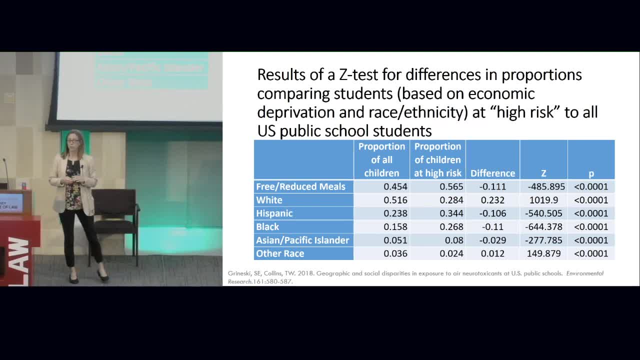 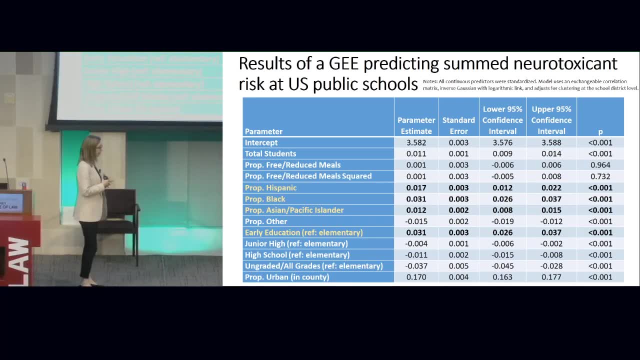 Then schools at lower risk or all schools, So this is just bivariate. We also took these data and put them in a multivariate model right, So we can look at, for example, the factors in the racial ethnic composition of the school controlling for the economic deprivation of the. 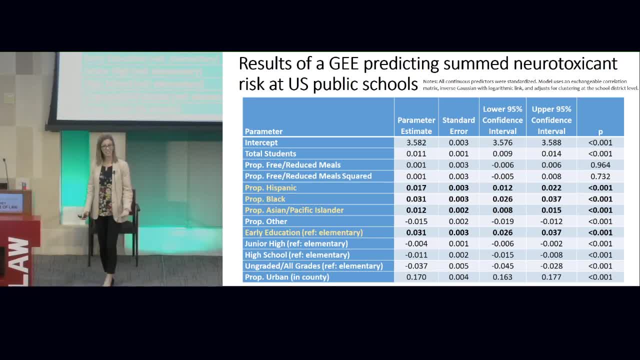 school, So we can separate race from income statistically. We can also bring in the level of the school, So whether the school is like a pre-K center or an elementary school or a high school, And that matters because younger children are more vulnerable to the effects of air pollution. Their brains are developing. their barriers are not as well developed as older adults. They're more likely to breathe through their mouth and therefore not get the filtering that happens when adults breathe through their nose. So there's many reasons why children, especially young children, are more vulnerable. 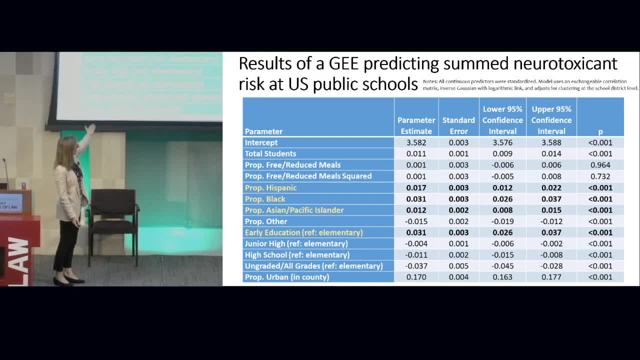 to the effects of air pollution. So we find in the multivariate model that as the percentage of Hispanic, black and Asian and Pacific Islander students in the school increases, the level of neurotoxicant risk significantly increased. And then we also found that early education centers. so the preschools, the Head Start centers, the pre-K centers also had higher levels of exposure than elementary schools. And then the older schools- not older schools, schools serving older children- had lower levels of air neurotoxicants than the elementary schools. 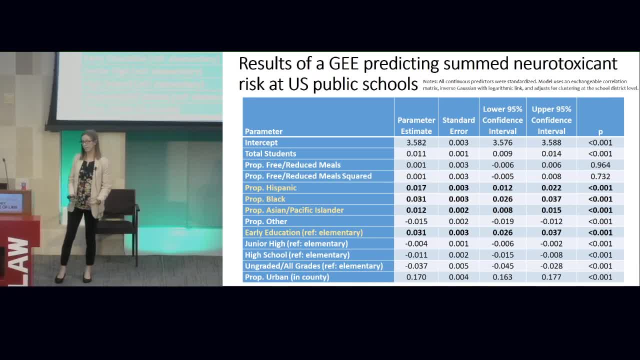 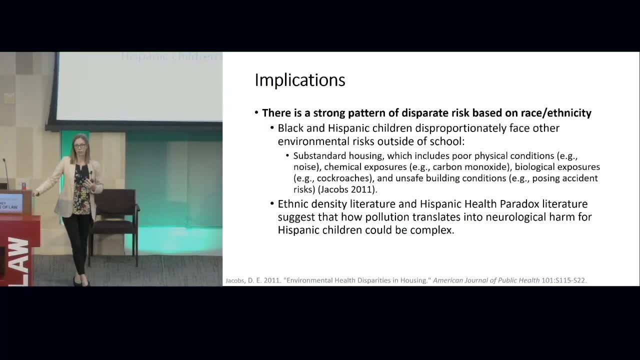 So we see schools serving younger children having higher levels of these air neurotoxicants. So the implications of this work one we see this strong pattern of disparate risk based on race and ethnicity. This is at school. There are many other studies showing risks. 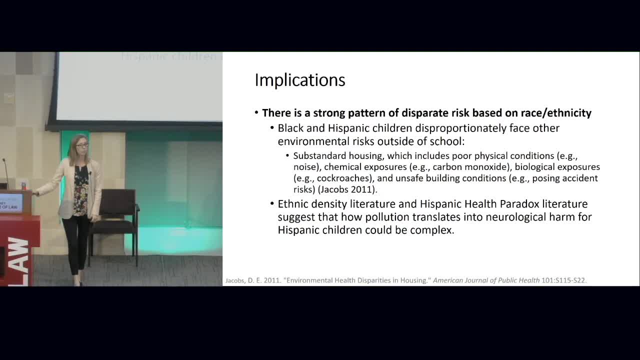 for black and Hispanic children. apart from this Right, They have higher rates of living in substandard housing, of chemical exposures, of biological exposures, of unsafe building conditions. There's many studies that show that they have increased risk of exposure to residential air toxins at home. 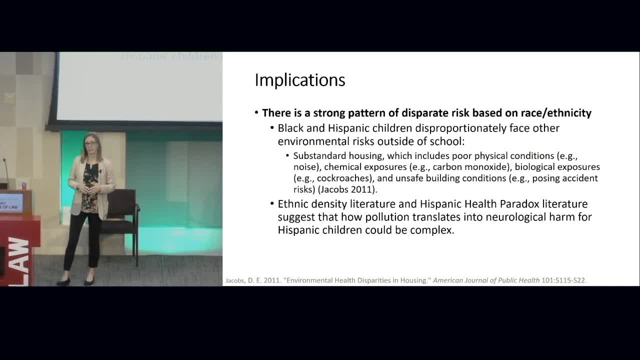 not only at school. So it sort of combines with the literature and demonstrates this pattern. There's some interesting work on the Hispanic health paradox. which is this idea? and that's not really an idea. I guess it's a hypothesis, although there's lots of evidence behind it. 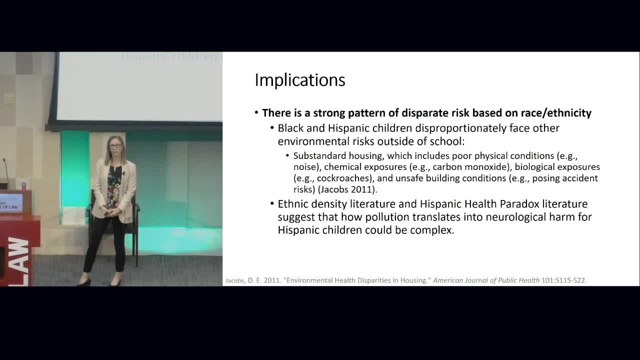 That, specifically, Hispanic immigrants are much healthier than you would expect, given their socioeconomic profile, And that the longer that they're in the United States that protective health effect erodes. But this group as a whole is much healthier than you would expect. 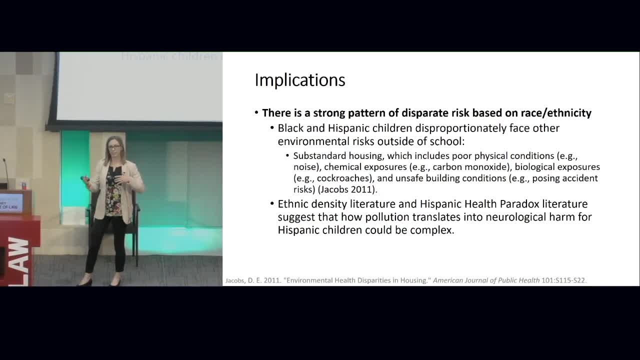 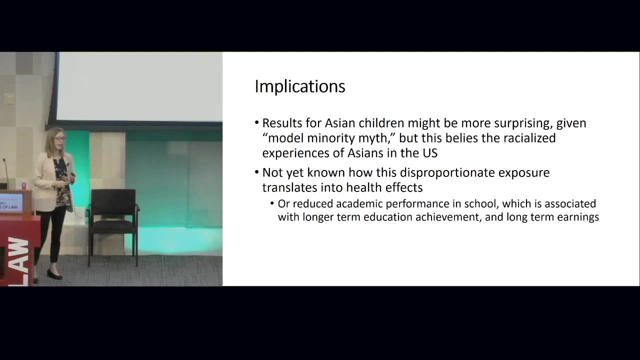 And so, when we think about these air neurotoxicants and this population, I think it'd be an interesting thing to investigate the effects on health and how- if at all or maybe not at all- that immigrant trajectory is protected. The study also highlights risk for Asian children. 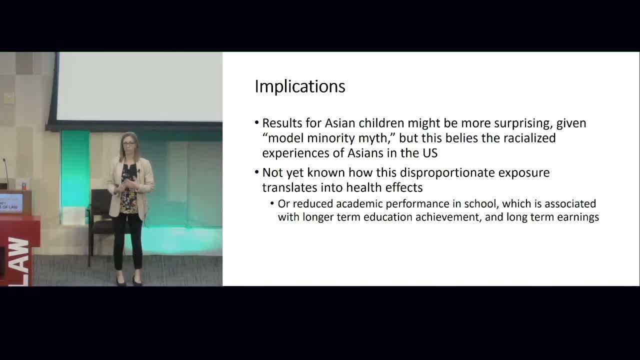 in the United States, And I think in general, people are a little bit more surprised by this finding because of what we call in sociology the model minority myth, this idea that Asian Americans as a whole have higher rates of education and higher incomes than whites. 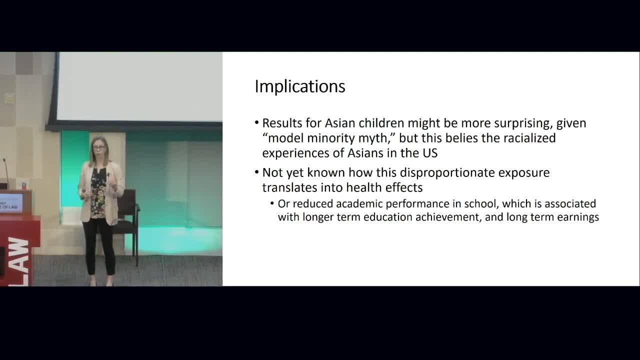 In sociology we call it somewhat of a myth because those statistics don't control for rural-urban differences. the Asian population in the United States is dramatically urban, where those things are higher in general, And also if we look at the Asian population divided up. 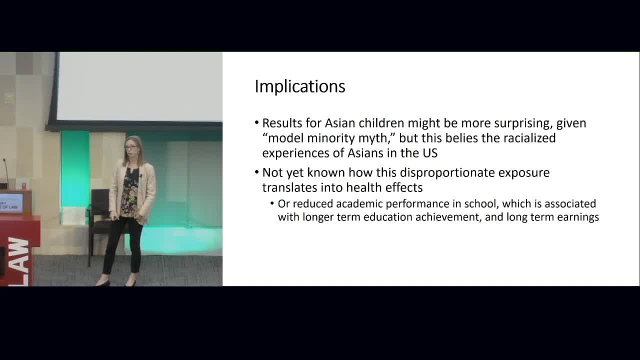 into different ethnic origin groups. they have dramatically different trajectories, And even high-achieving, well-educated, rich Asian Americans face substantial discrimination in the United States in interpersonal relationships and also at work. So it's not totally surprising, but in some ways 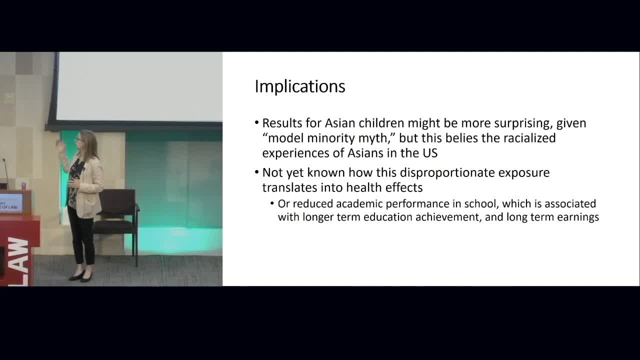 it seems surprising Now. at the time in which we wrote this study, it was sort of unclear still what the effects of this disproportionate exposure might be on health effects and academic performance. Since the study was published, several studies have come out that look specifically at this, which? 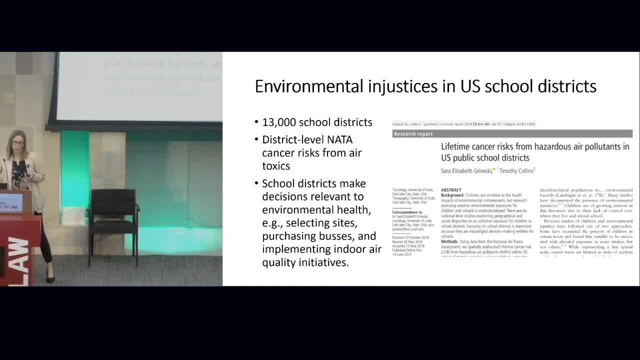 I'll get to in a few moments. So the attention that we got from that study from states Department of Environmental Quality contacted me. NPR, The Guardian, just different People were really interested in this work And so I got to thinking: what else? 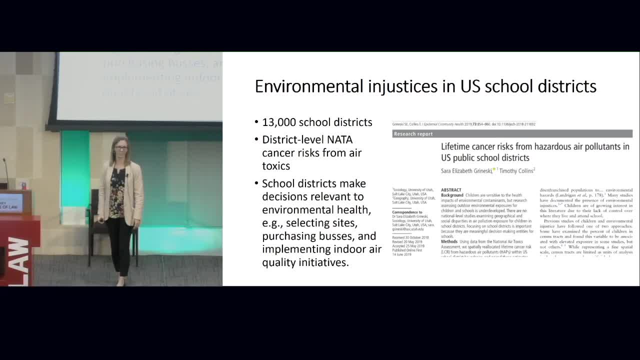 could I do? that might actually make an impact, Because you write so much stuff and no one ever reads it right. So this seemed to be something that people are interested in that maybe could contribute to policy discussions about air pollution regulation in the United States. 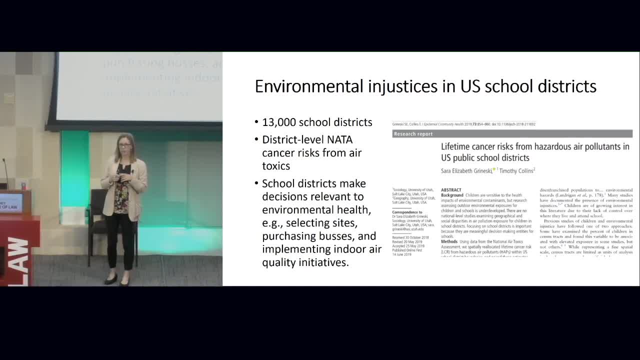 So we did a follow-up study looking at school districts, Because what I realized from the work on schools is that individual schools don't have a whole lot of power in terms of regulating their environment. They're governed by a school district. School districts, on the other hand, 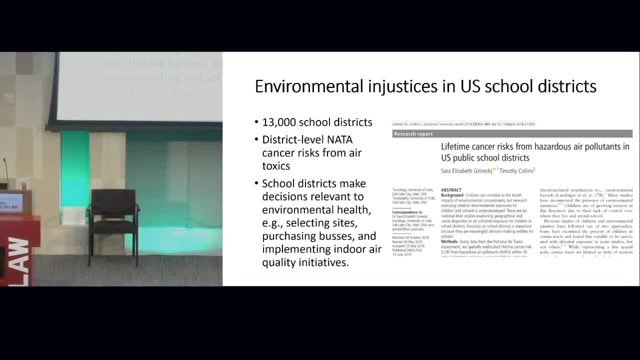 are the ones who select sites for building schools, make decisions about closing schools, purchase school buses- which, if you know, school buses are a huge source of air pollution around schools, especially when they're diesel, And the school district is also able to implement. 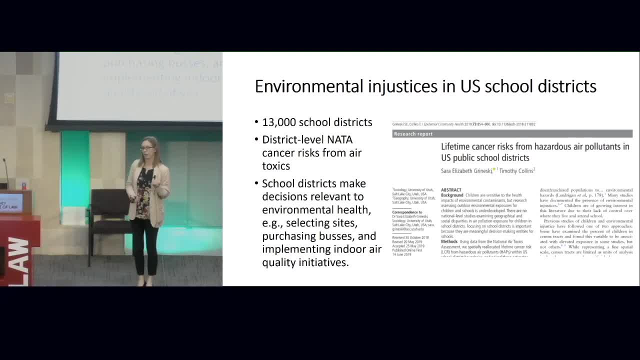 for example, indoor air quality initiatives that affect children's environmental health. So it seemed to make sense to look at school districts And here, instead of doing that, my air neurotoxic index, I just used the cancer risk. This is the cancer risk measure, which. 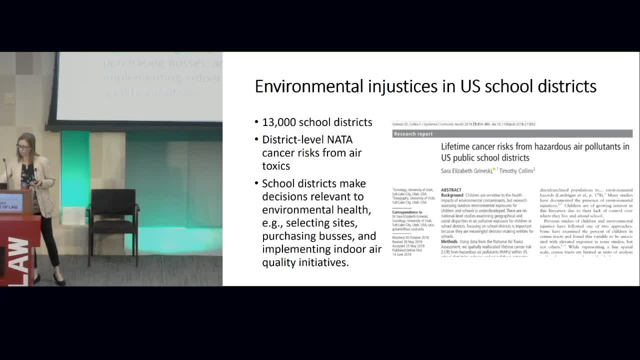 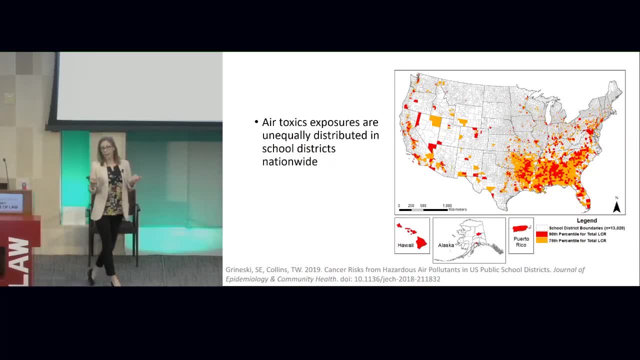 is a much broader, general measure of air pollution exposure. This is a map of all the school districts in the United States. There's roughly 13,000 public school districts in the United States. The red school districts are in the top 10% for cancer risk. 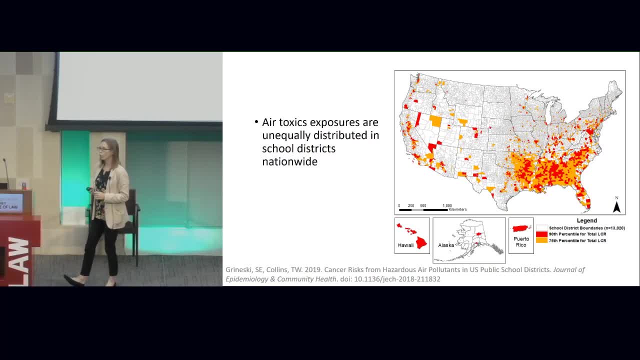 due to the exposure of hazardous air pollution in the neighborhood. The orange ones are in the top, between the 70% and the 80%. Here in Utah you see we have some red and orange school districts: The red blob in Utah, the red blob at the top. 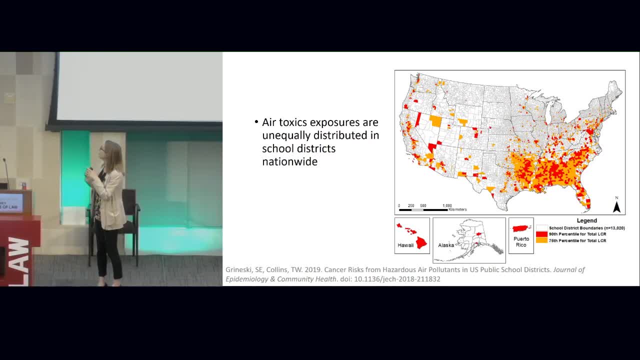 is Granite School District and Salt Lake Independent School District. The orange below it is Alpine School District And that bright, red tiny circle in the middle of Alpine is the Provo School District. So we do have school districts here in the metro area that rank very highly nationally in terms of their risk. 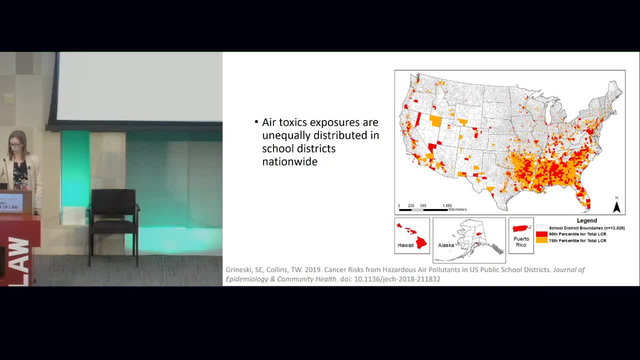 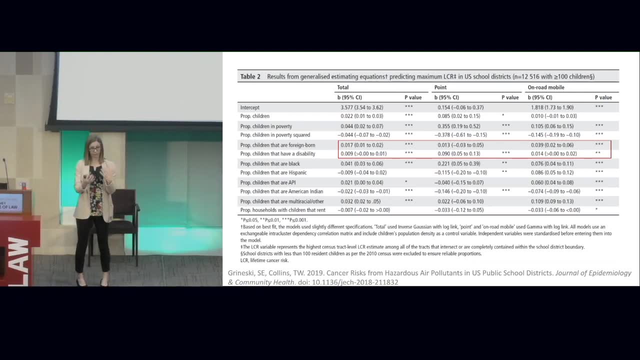 And that's due to hazardous air pollution exposure. We did a similar analysis in this paper, a multivariate analysis where we included a bunch of different variables predicting exposure to these cancer-causing air toxics. We found racial, ethnic findings, as we did in the previous paper. 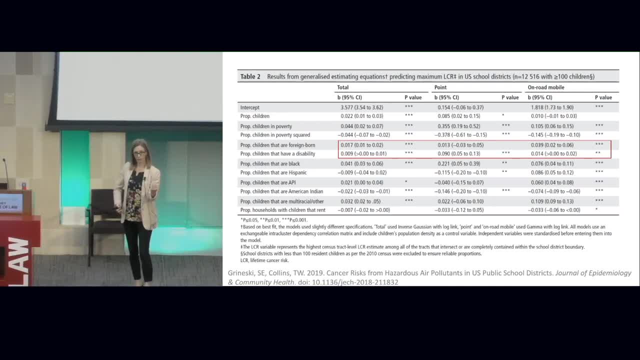 But what we added with this one- because I wasn't reliant on school data but I could use census data for the school district- was that schools with higher proportions of foreign-born students, and so schools with higher proportions of disabled students, had increased risk to these cancer-causing air. 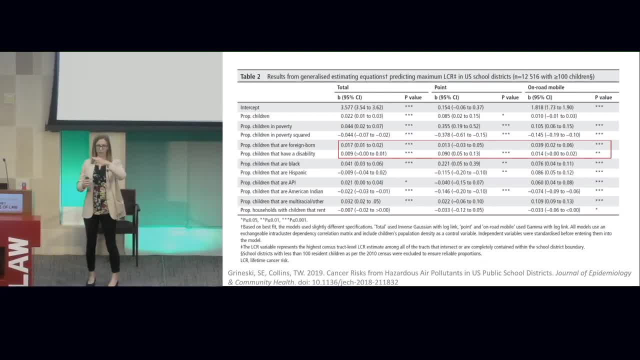 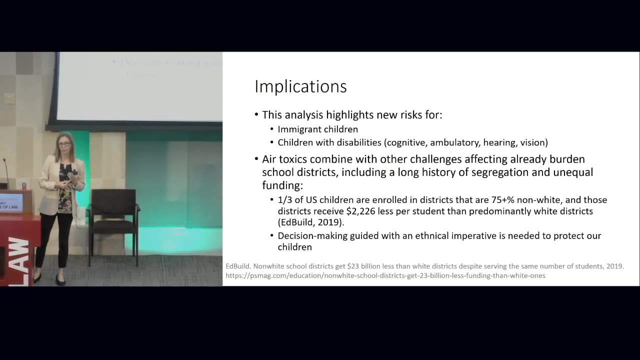 toxics in the school district. So I'm looking specifically at the composition of the school district using census data and the NATA measure at the school district level. So the analysis highlighted the risk for immigrant children as well as children with disabilities. 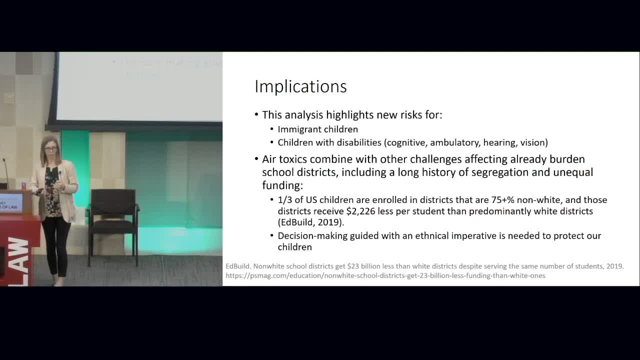 And the doing it at the school district level brought me into some of the research and some of the literature on the history of school segregation in the United States, And there was a recent report that just came out earlier in 2019, and it showed what a lot of us already know. 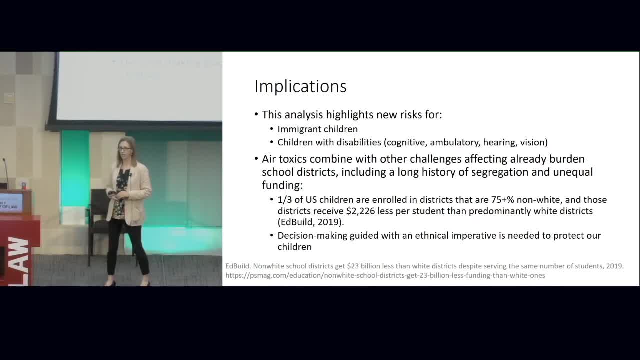 these dramatic differences in school funding based on the racial ethnic composition of the school district. So this report showed that a third of US children are enrolled in districts that are more than 75% non-white, And that group of school districts received $2,226. 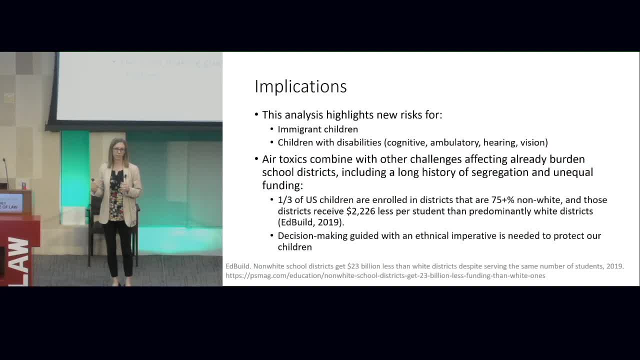 more per student than the districts that are 75% or more white. So we see that this air pollution exposure is combining with other challenges that school districts are facing, especially school districts that are serving racial, ethnic minority students, And this analysis definitely speaks to this idea. 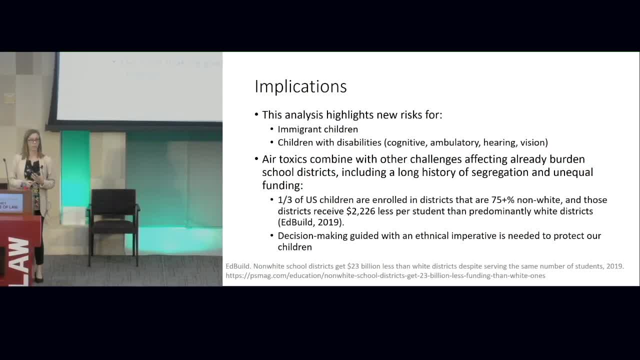 that we need to think more about children and their well-being as we make decisions about where to put our schools and how to allocate resources at the school district level. All right, That brings me to this, I guess second to the last part. 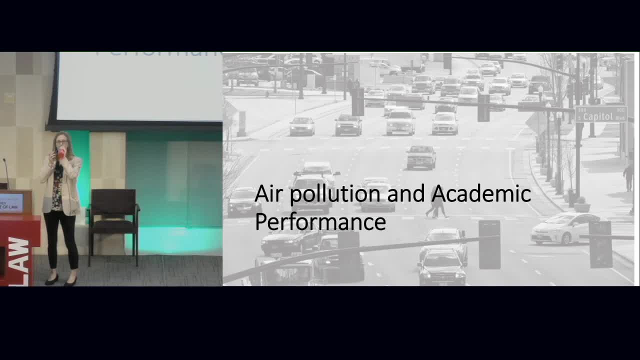 of my presentation on air pollution and academic performance, And I will begin by telling you that when we decided to write our first paper on this topic, I was working with a- then, I guess, senior undergraduate student who was going to enter the graduate program. 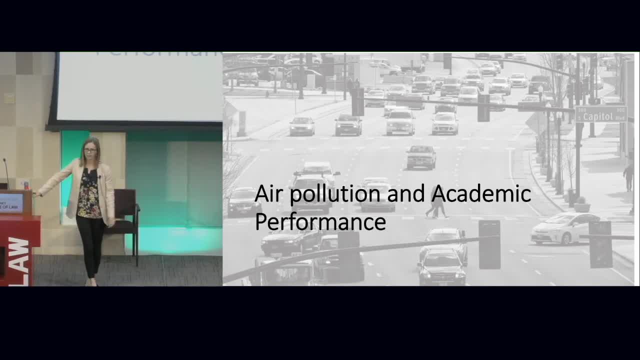 And she was a single mother and she was interested in kids And we had this data that we could use to look at the effect of school-level air pollution on GPA. And I remember sitting in my office with her saying: you know, Stephanie, this just. 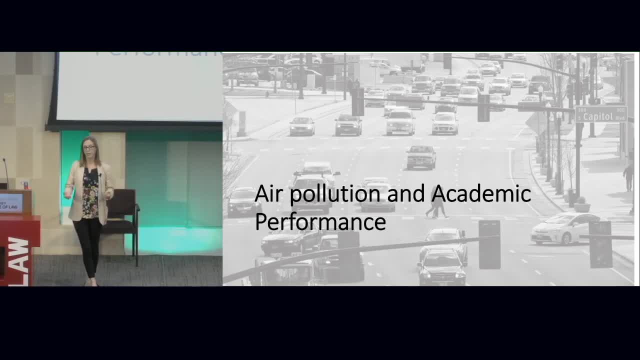 might not work out. There's so many things that impact GPA. We were doing this work in El Paso, where many children struggle with English language skills when they enter the elementary schools, And there's a lot of families in poverty, And I was like I just don't know if we're 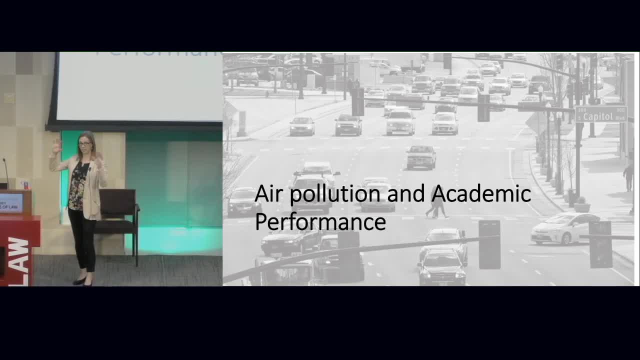 going to find anything, Stephanie, But sure we can try it. And then it ended up being the strongest finding that we couldn't make go away. So it's kind of interesting. So what do we know today about this topic? All right, 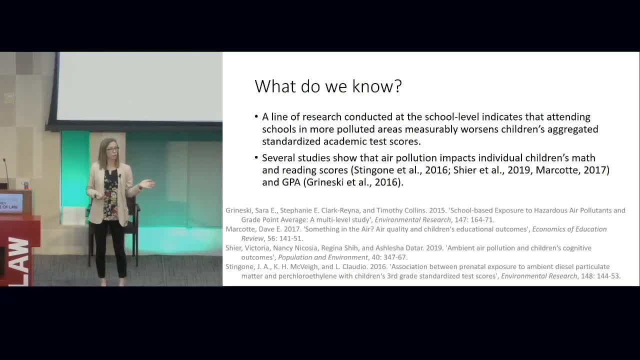 Let's talk about this topic. There's a line of research that was conducted as early as the early 2000s, looking at the level of air pollution at a school and the standardized test scores aggregated of all the students in that school. Many of these studies were done in California. 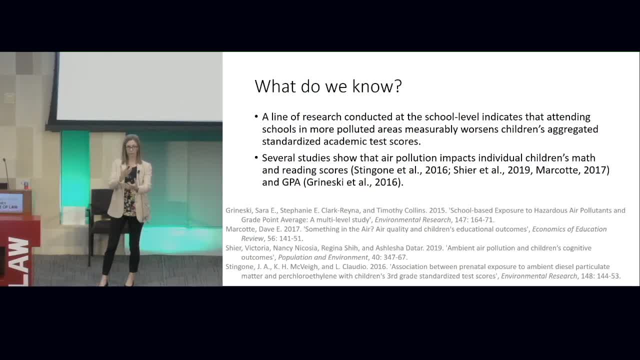 There was also work in Louisiana and Michigan And these studies found that controlling for school demographics, that attending schools in a more polluted area, worsened the standardized test scores of the students in the school, And then in very recent years we started to look at the level of air pollution. 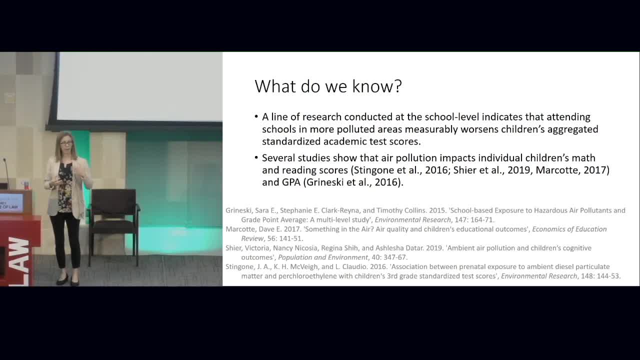 in the school And in recent times a few researchers started to look at individual kids and how air pollution exposures influence their academic skills. So a couple of studies came out very recently looking at math and reading scores. And then we did this study looking at GPA. 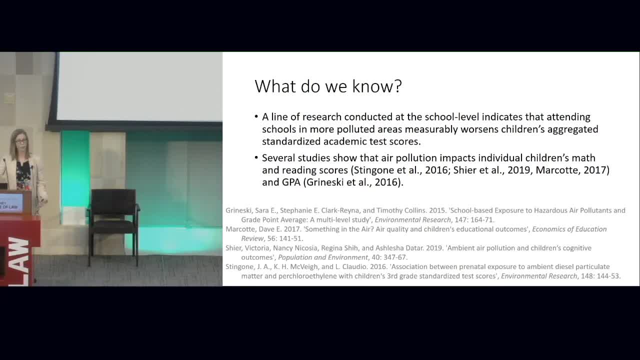 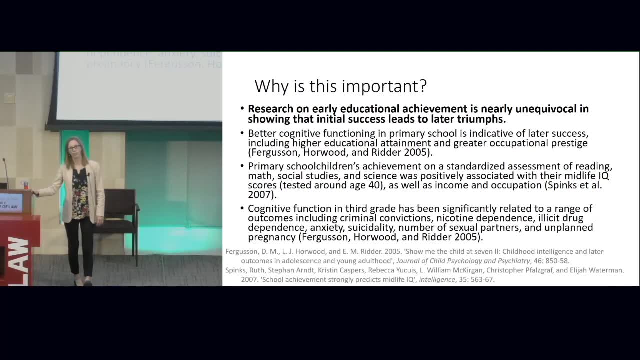 but actually looking at individual kids instead of just this aggregate school level approach, both of which are important. So why is this important? There's many reasons why this is important. I'm not going to go into all of this, But it's worth peeking at least briefly. 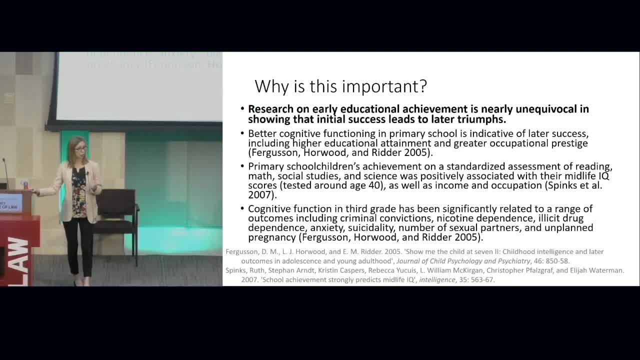 at the literature that documents how important early school performance is on trajectories into adulthood. The literature is nearly unequivocal that initial success leads to later triumphs. So better cognitive functioning in primary school is related to educational attainment, greater occupational prestige, higher income. 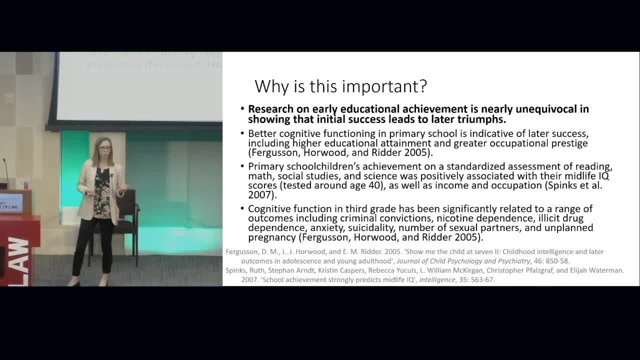 Primary school achievement was related to midlife IQ, as well as income and occupation, in another study. And then this study looked at all of these things that we tend to think of as negative and found that children's cognitive abilities in third grade were related to all kinds of things. 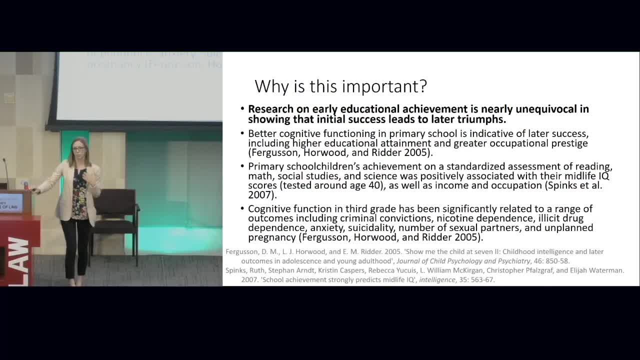 in their future lives, whether they were addicted to smoking cigarettes, whether they used illicit drugs, whether they had unplanned pregnancies, all kinds of thing. So I think that this research, plus just what we already know, underscores the importance of thinking about primary school. 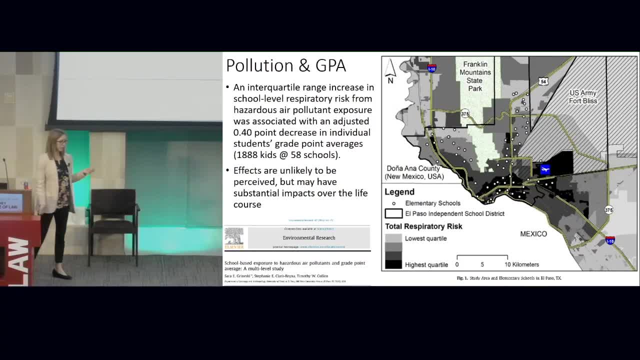 children's school performance. So I mentioned to you the study that we did in El Paso. We did a survey of about 1,900 kids in the El Paso Independent School District And the survey was largely focused on respiratory health. But we were aware of those studies in California. 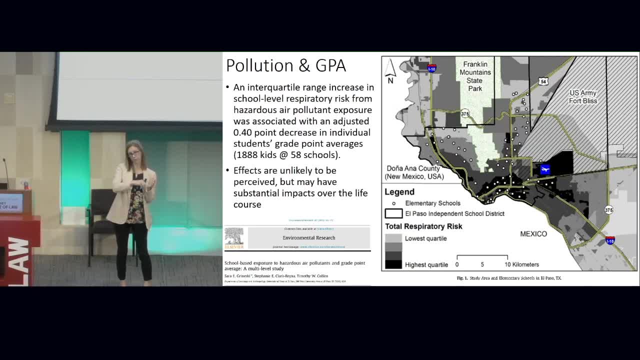 finding that association between school-level test scores and pollution. So we randomly threw on a few questions about how your child was doing in the five subjects that the EPISD has on their report card. OK, So we ended up using those data. We did this study. 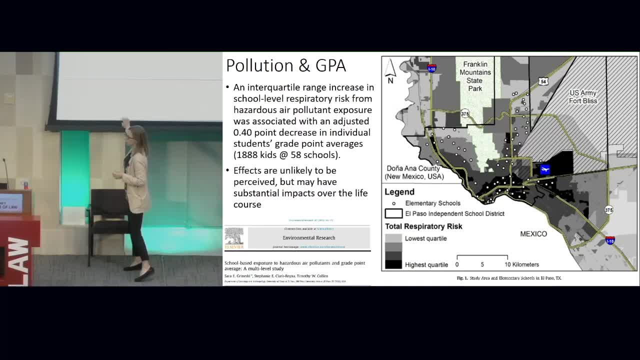 And we found that, depending on- we did several different studies- The one I'm highlighting here is school-level pollution. So the level of pollution at the school was associated with an increase in the pollution at the school was associated with a decrease in the child's GPA. 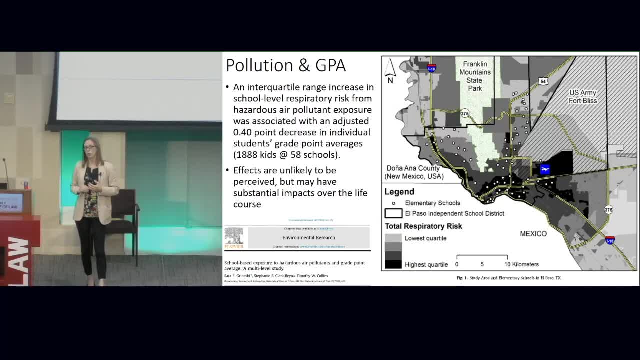 based on these five subjects on the report card. So we got to thinking about this And we realized- and at this time I also had a young child And it was like how would you even know? how would you even know that the air pollution is? 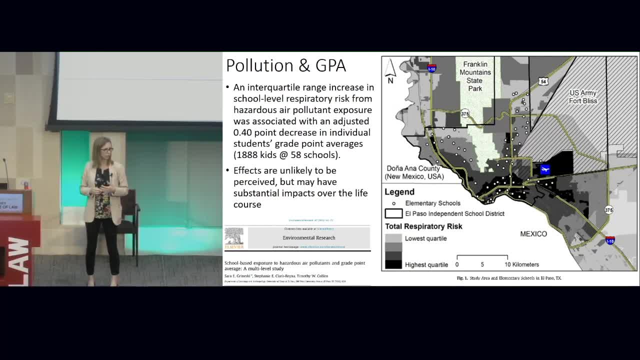 making your child not do quite as well in school as they would if they were living somewhere else. Like it's very insidious, Because I don't know how you would ever know that your child should have been smarter, but they aren't. 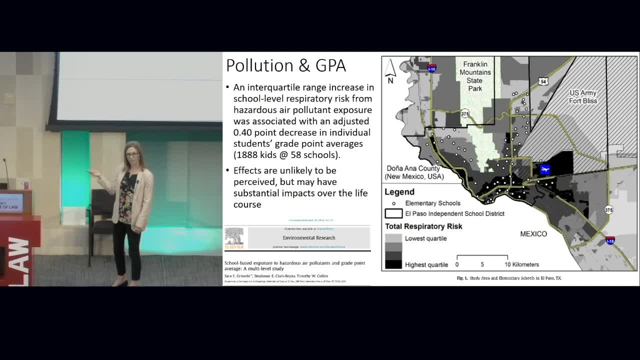 You would never know. So these effects are very unlikely to be perceived, And I think that means they're unlikely to bring us to any sort of action, Because unless we have research that aggregates it like this and shows this to us, it's hard to know. 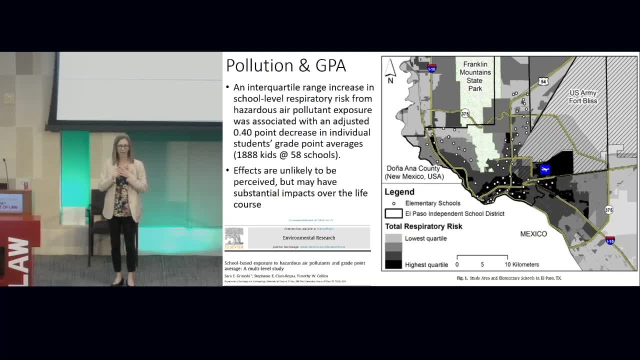 where if your child goes outside to wait for a bus and starts having an asthma attack? like you see, the bus is making my child sick. This is much harder to see, which I think makes it harder to address, But certainly it means that this could have impact over the life. 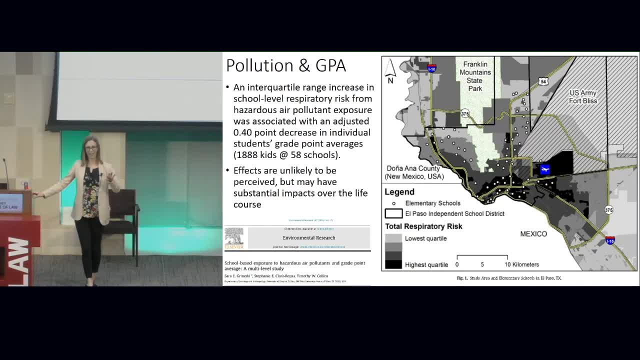 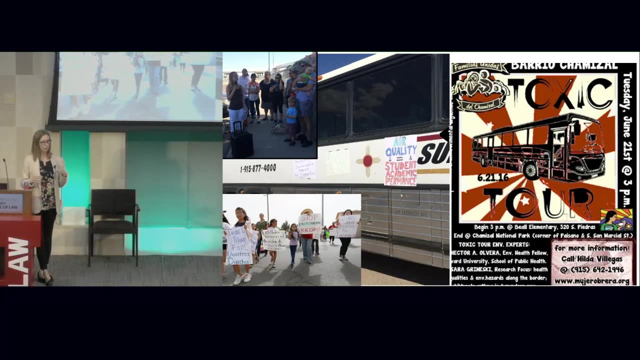 course, given the research I just presented to you about the importance of early academic achievement on later success. So this study led us to become involved with a community group, Familias Unidas de Chamizal. Chamizal is a neighborhood located right. 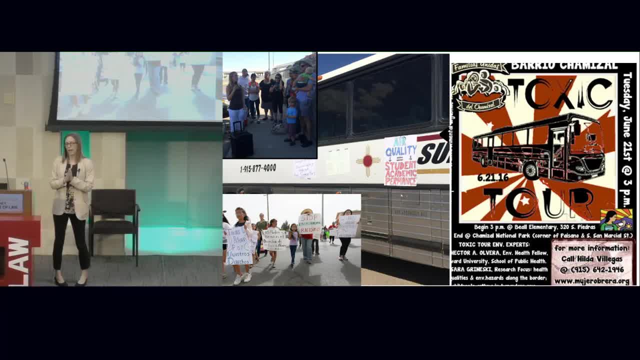 next to the US-Mexico border in El Paso, They have three of the most polluted schools in the EPISD, And so they were really interested in this study, And there's been a lot of talk. It's still ongoing. This picture I just grabbed from last week. 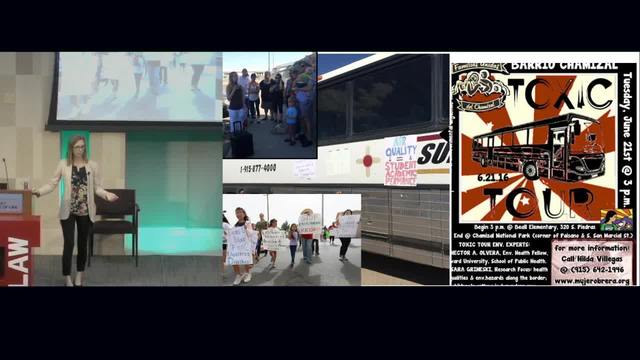 talk about closing the schools in this neighborhood due to declining population, not due to the environment, But a benefit of that will be the reduction of children going to school in really polluted spaces. But the parents are trying to decide which of the schools they should keep open. 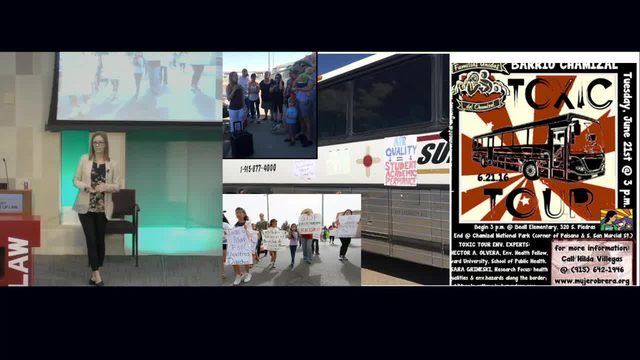 And the school district has their own views, And so it is the case that the raw data from our study is being used in these discussions about which schools are most polluted. But they did a toxic tour in a big bus, And I think it'll be the only time ever in my life. 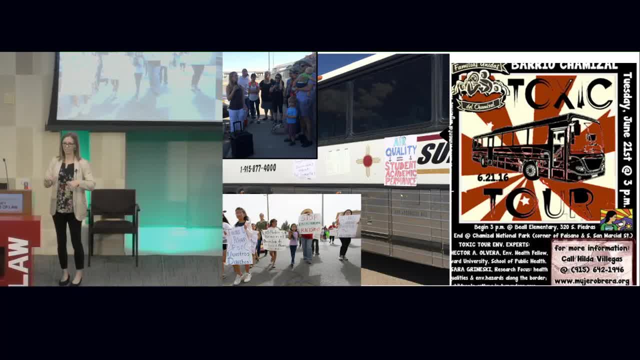 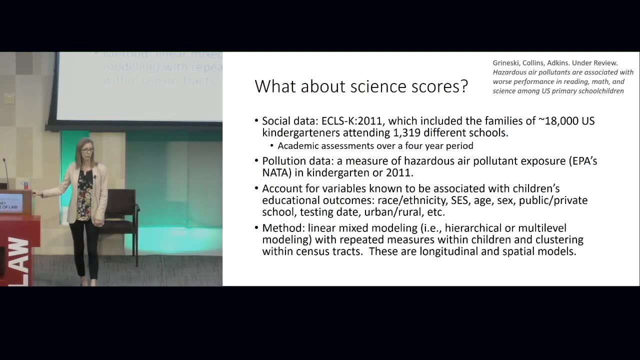 that my research is on the side of a bus. Air quality equals decreasing student academic performance, So part of that issue is still ongoing in El Paso now. So the newest work that my team is doing in this area- it's still under review. 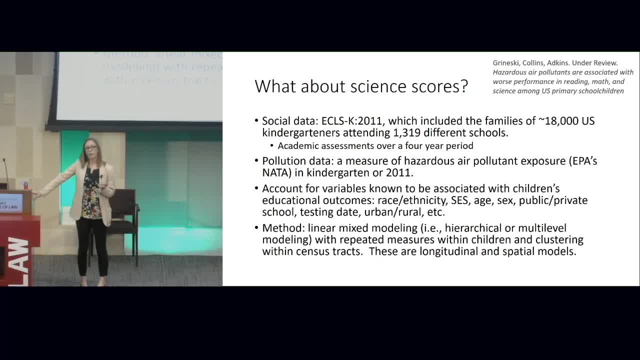 We have a second set of revisions which I'm submitting tomorrow. But we look at reading and math, which other studies have done, But we also look at science which hasn't been examined yet in this context. So we're using a national level data. 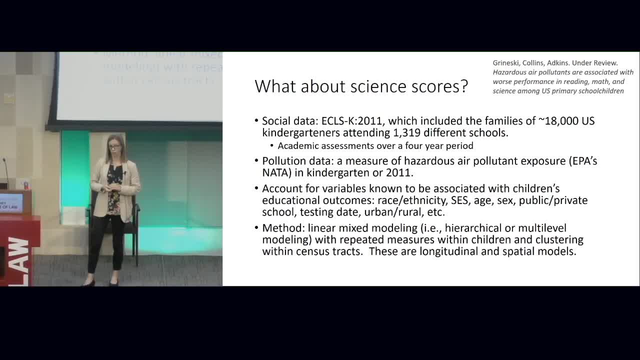 set of 18,000 US children attending public and private schools. They entered the study as kindergartners and they stay in the study through fifth grade And they do these direct academic assessments, Where this trained team of researchers comes in and tests the kids in reading, math and science. 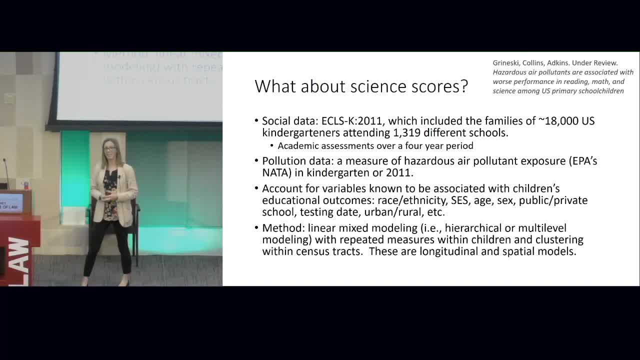 in the fall and the spring throughout their elementary year. So the data is very high quality for this type of work. And then this is just sort of we're getting started. So we used the NATA again because 2011 is the year in which these kids are in kindergarten. 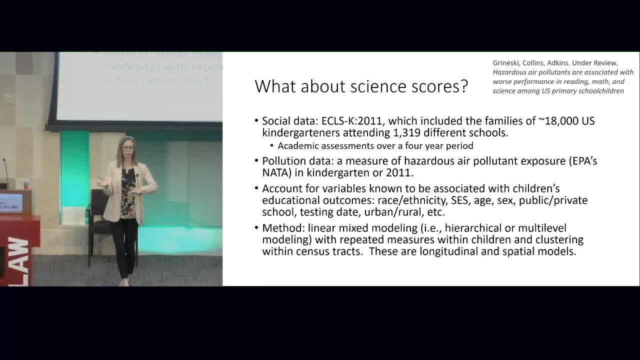 So it provides a measure of exposure when they begin school. Of course, we don't have exposure before they started school, which is a limitation, But we're able to measure the pollution exposure and we're able to measure when they began school. 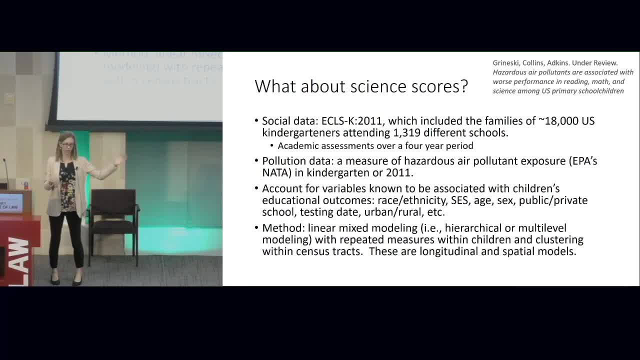 And it's worth saying here that we try to control all these studies, including our study in El Paso, try to control, for all the other things that we know impact children's academic performance, Their parents' level of education, the race, ethnicity, whether they're young or old in the grade. 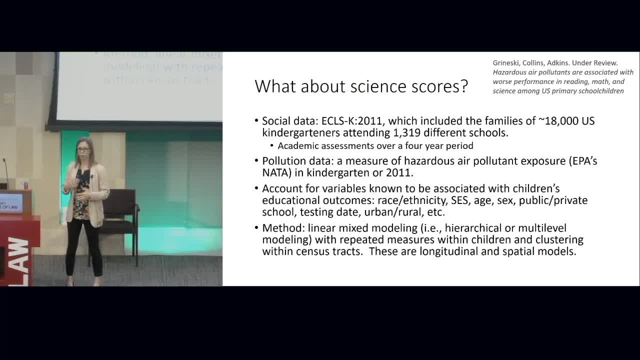 if their family speaks English at home, if they're in an urban or rural school, public or private school, if they were tested, in this case earlier versus later in the year. Like we try our best to account for all the other things that. 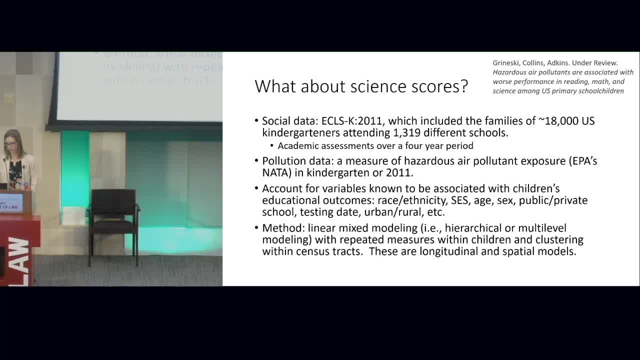 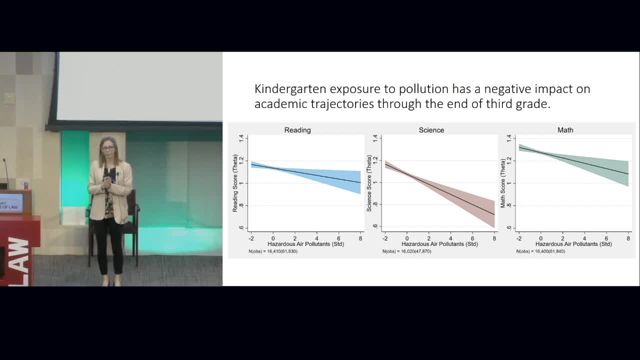 are known to be associated OK, So we're able to do that with students' academic performance. What we find in this work is that kindergarten exposure to pollution has a negative impact on academic trajectories to the end of third grade. So because we have these repeated measures, 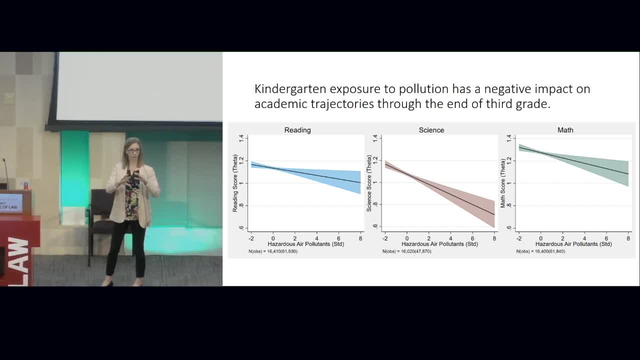 of academic performance. we look at the kids' scores in kindergarten, in first grade, in second grade and in third grade And you can see that there's a negative slope, which is what you would expect: More pollution, lower scores. 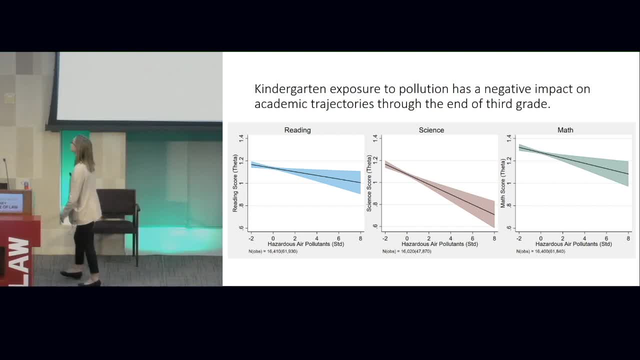 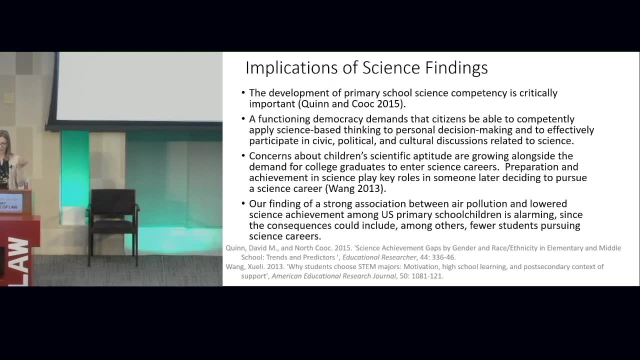 And this is controlling for those other variables that we know are associated with it. But performance, You see, the slope is the steepest for science, which means it has the strongest effect. So, because math and reading have been examined before, they're certainly very important. 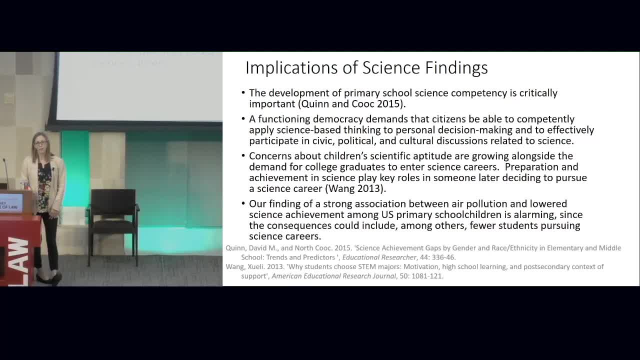 I'm going to just talk briefly about the science finding. So you probably know right, the development of competency in science in elementary school is very, very important. You hear about the shortage of STEM professionals in the United States. Back in the Obama presidency they 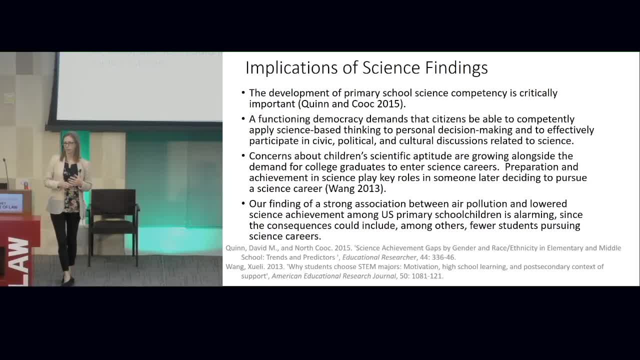 called for a 33% increase in the number of people entering science careers. Democracy requires people that can competently apply science-based thinking to decision making to participate in the policy process, But this is very important, And so we already have concerns about science achievement. 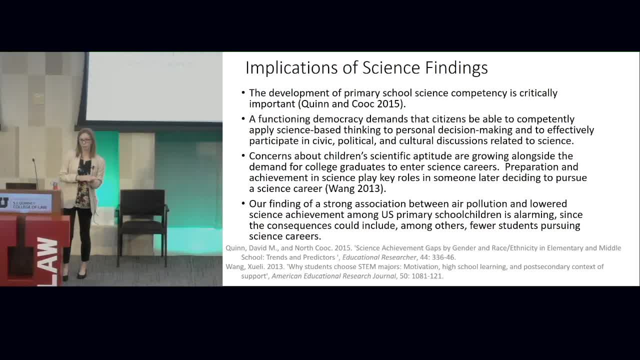 in the United States, And I think this finding of this relationship between air pollution and science achievement is alarming And it could have consequences for the future in terms of our scientific discovery If we're taking away from people's abilities to live out their human potential. 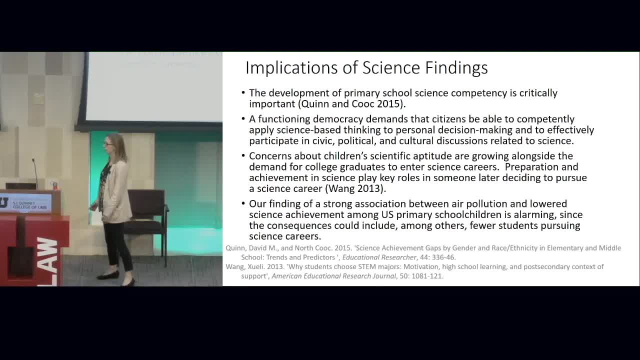 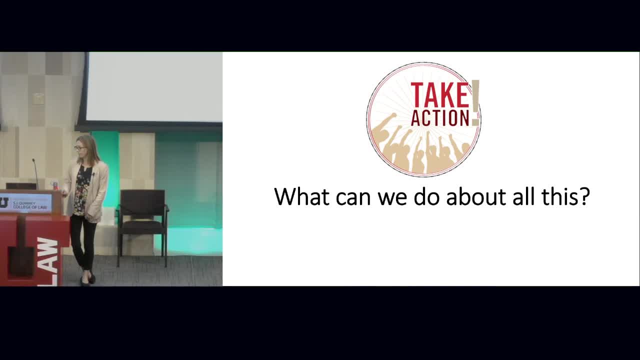 by exposing them to air pollution. it's pretty concerning and pretty alarming. What can I do about this? I do not have all the answers, That's for sure. It's something I definitely think about And I think it's something that requires conversations. 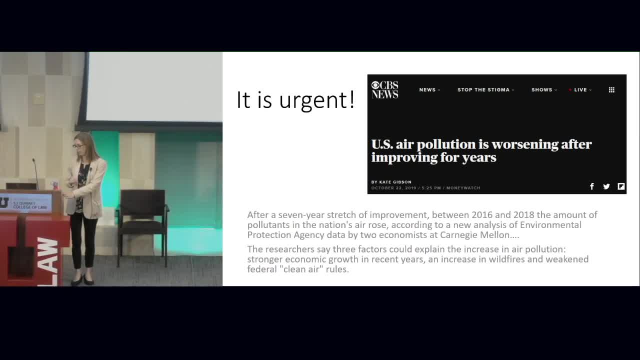 I will say that it's pretty urgent. I don't know if you've seen the news in the last couple days. This is from October 22.. That's yesterday, two days ago. The US air pollution is worsening after improving, So in general we've seen a nice. 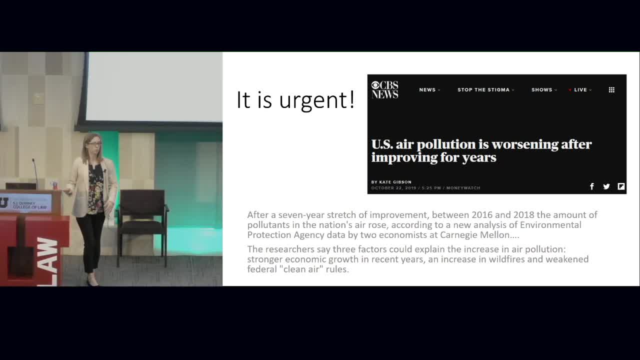 nice improvement in our air quality in the United States. This article is specifically talking about how, after seven years of improvement, we've had a decrease, But the trend actually goes back several decades beyond that. A lot of us think the air quality is getting worse. 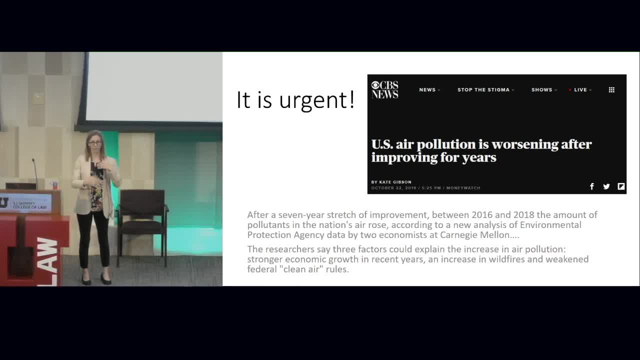 But the PM standards, for example, have been getting more restrictive, giving us more bad air days, even though our air is actually better, And that's a general trend in the United States and also here in Salt Lake. So currently we have concerns about our air pollution. 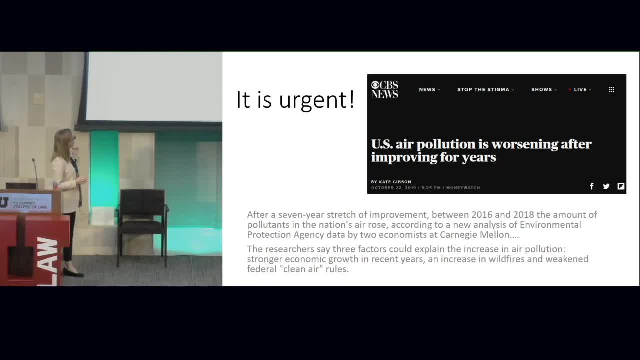 It's getting worse And these researchers from the Carnegie Mellon related it to economic growth, all the wildfires that we've been having in recent years and a weakening of our federal clean air rules, as well as increasing lack of enforcement of the existing clean air rules on the books, 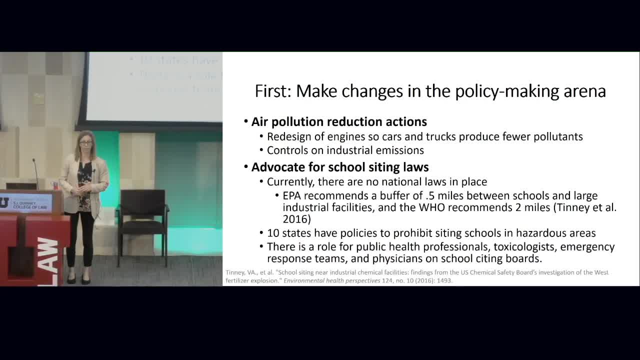 So clearly air pollution reduction is really important. If I look back at the history of the United States in terms of our reduction in PM 2.5, you can clearly see that controls on industrial emissions and the improvements in our automobile technology have had a dramatic impact. 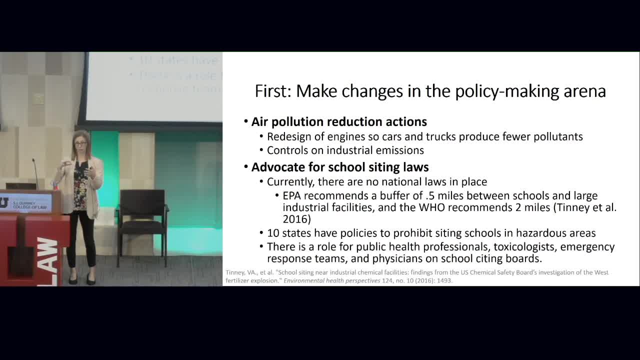 And so clearly we need to continue to innovate in those areas And I believe also at a federal and state level sort of force, that innovation through policy that is restrictive. Then we don't actually have any laws in place that say you can't put a school next. 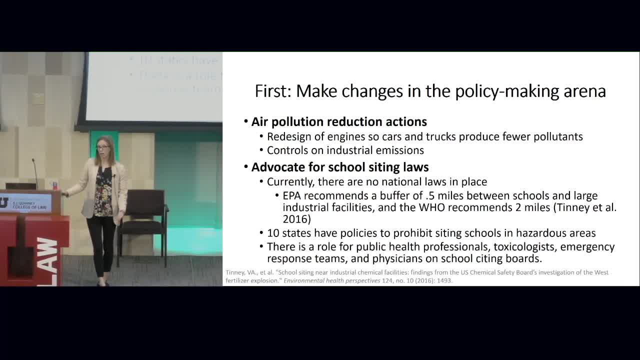 to an environmental hazard. So there's no national law. There's also no governing body in charge of the location of schools. So there are some recommendations. The EPA recommends a buffer of a half a mile between schools and large industrial facilities. The World Health Organization also has guidelines. 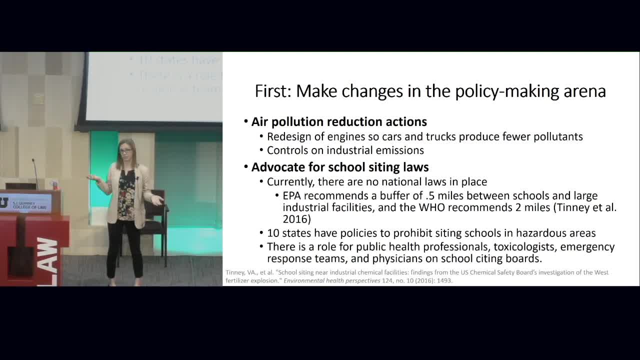 and they recommend two miles. But this is recommendations, right? There's no law in place. 10 US states- and I believe Utah is not one of these 10, have policies to prohibit school siting in hazardous areas. So at the state level, 10 states have said. 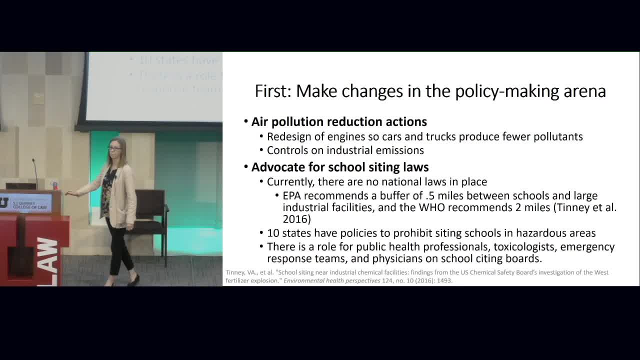 OK, we're going to do something about this because it's a concern And as we think about school siting, that brings me back to the focus on school districts. right And often, the composition of school boards does not always involve public health professionals. 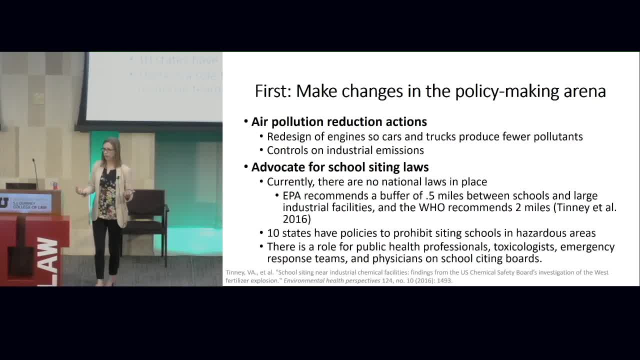 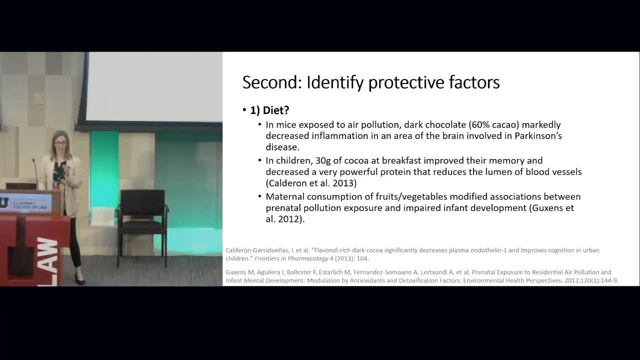 toxicologists, emergency response professionals, medical doctors, right. So as we think about siting schools, it seems like there's a time to sort of broaden the conversation and bring in different experts who will have additional knowledge about school safety. So another thing I'm interested in: 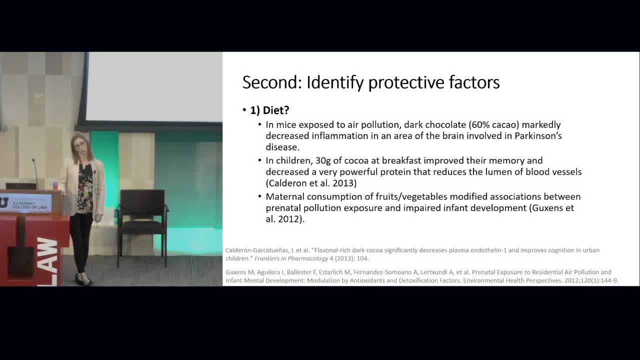 because I worry that I don't know how fast the air is going to improve. I hope that we can enact these policies that will better protect children, but I'm not sure. So one of the things that our team has been thinking about is what might be some things that would protect kids. 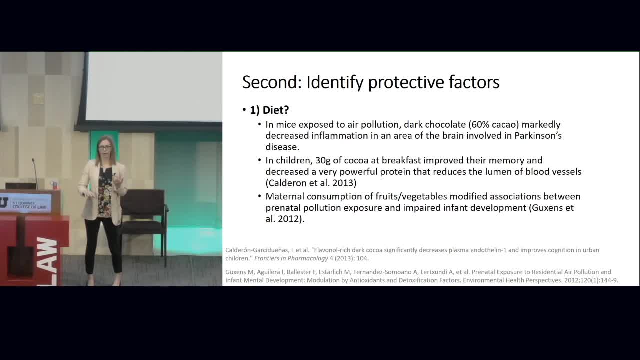 So we know there's this relationship between air pollution and reduced cognitive ability, economic performance, But are there things that we could do at the level of the family, at the level of the school, at a level where maybe it's a little bit easier to enact? 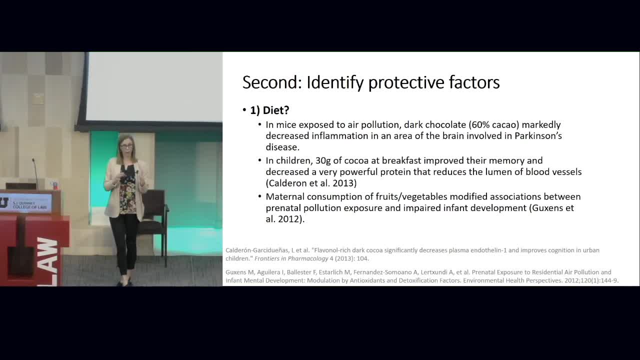 So we've been looking at the literature to try to find what are some of these factors that might be related, And I don't have the answers for you. This is an open research question. It's a proposal I have into the NIEHS right now. 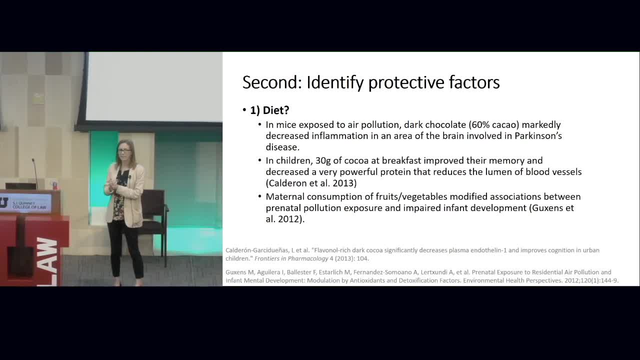 But the question is: would diet? is there anything that we could eat that would protect our brains in some way? The same person I mentioned earlier, the woman at the University of Montana, Lillian Calderon. she's done some work on chocolate. 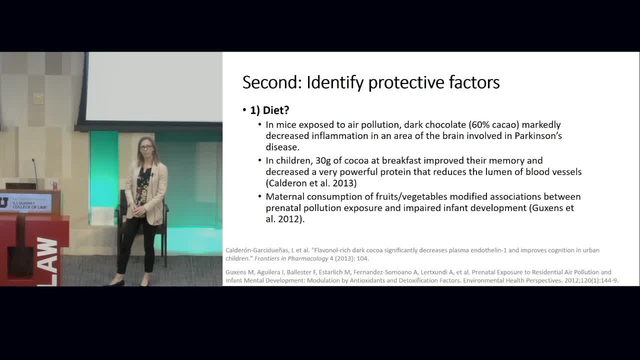 and how dark chocolate decreases inflammation and maybe somewhat protective when we think about cognitive decline and air pollution. There's also been a study that showed that the more fruits and vegetables that a pregnant woman ate while pregnant reduced the negative effect of the prenatal pollution exposure on the infant development. 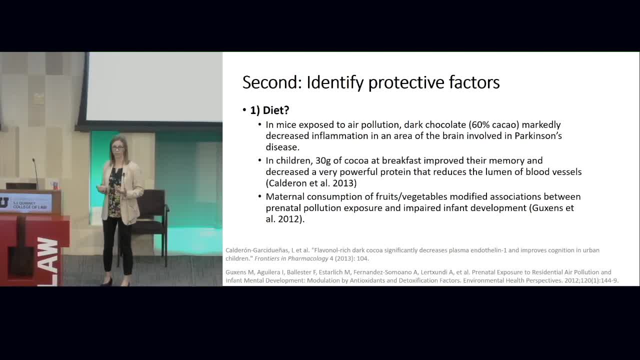 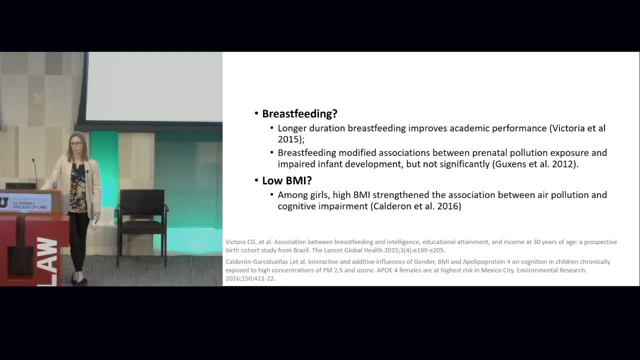 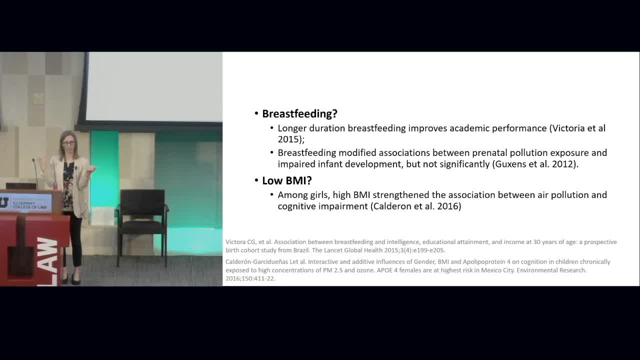 DR LILLIAN CALDERON MD. Yeah, So that's another modifier of relationship between prenatal exposure to pollution and infant development. They found a relationship But it wasn't significant. But again, this has been investigated so little. 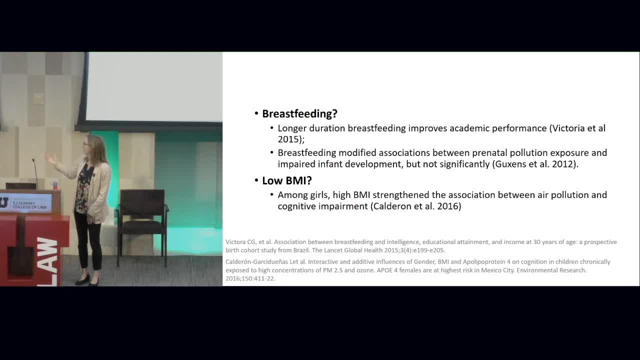 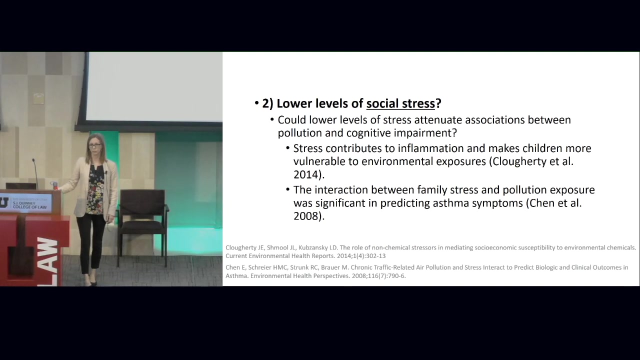 it seems like something one could look into. Dr Calderon again has looked at BMI And she found that amongst girls, having higher BMI made the relationship between air pollution and cognitive impairment stronger, which means that lower BMI make that relationship weaker. Then there's the pathway of social stress, right, Could lower levels of stress attenuate this? 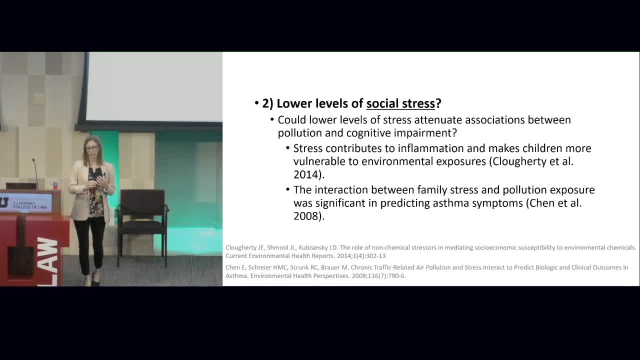 relationship make it a little bit weaker. There's quite a bit of literature in the area of air pollution and asthma that show that stress makes that association stronger. So kids that live in a home- for example the Chen study- where there's a lot of stress, the pollution is more strongly. 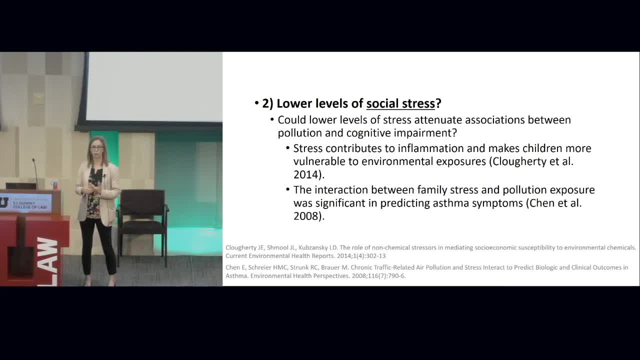 related to their asthma symptoms than when they live in a family with lower stress. So there's actually quite a bit of research looking at stress as a mediator, not so much in the academic performance literature, So I think it's a good hypothesis. Then I'm interested in the idea of 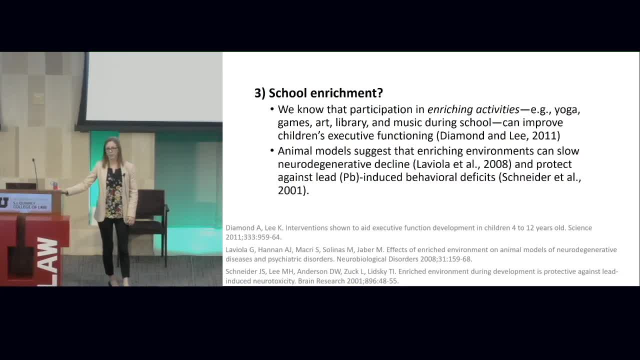 what could we change at the level of the school? So there was a study published in Science back in 2011 that showed that enriching activities like yoga games, art, going to the library, having a school music program improved children's executive functioning. having nothing to do with air. 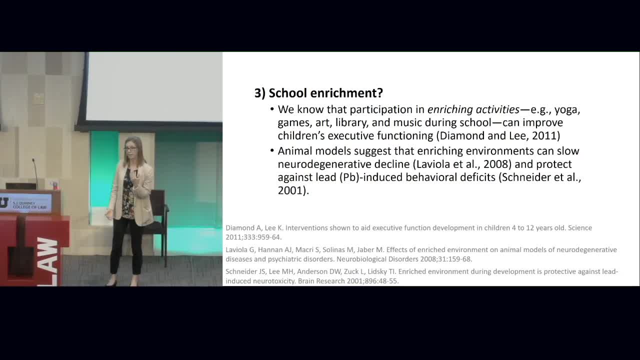 pollution, right. Just those things made their executive functioning better. And then I found a few studies looking at animals right that found that putting the mouse in an enriching environment slowed the neurodegenerative decline from exposure to lead. So maybe there's 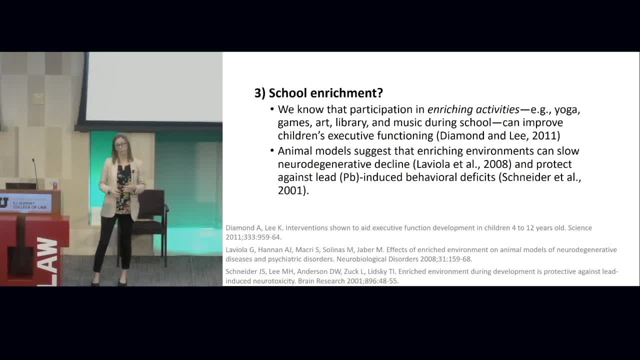 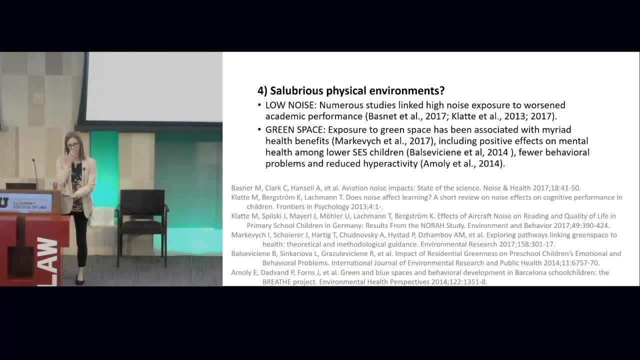 something about schools. if schools can be more enriching, that may be able to protect children a little bit from this sort of decline. And the last factor that our team is interested in examining is other physical environmental features, So noise, for example. 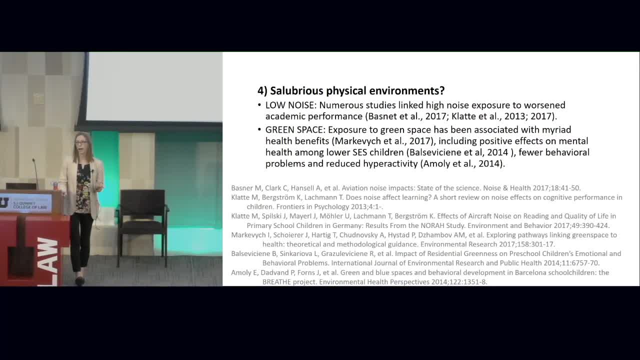 and also green space. There's so much literature on the health benefits of green space In kids that have, especially at the school level. the studies have been pretty strong that school level green space is good for kids' cognitive functioning, So I don't know if it could possibly interact with. 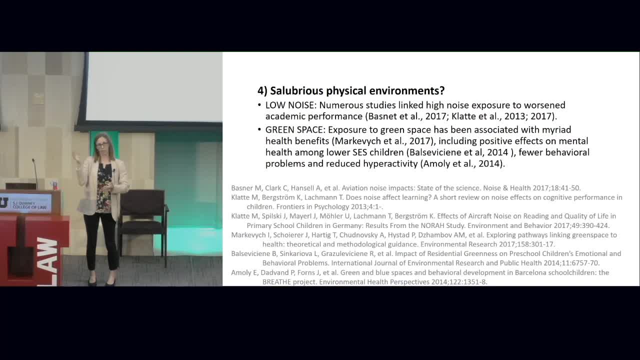 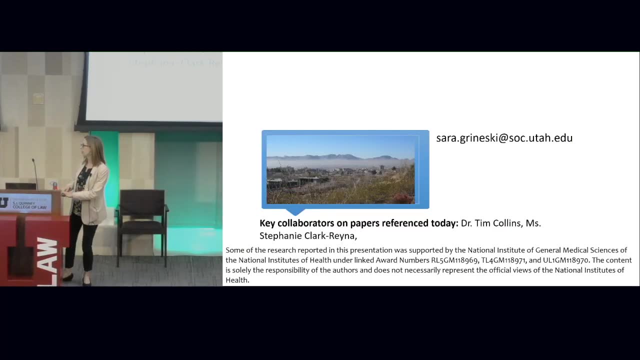 pollution in a positive way. Certainly, the green space trees help reduce air pollution, So it's something that is worth considering. I'm sure there are many more. Those are just sort of our current ideas, And that brings me to the end of the talk for today. So, as you notice from the citations, the key 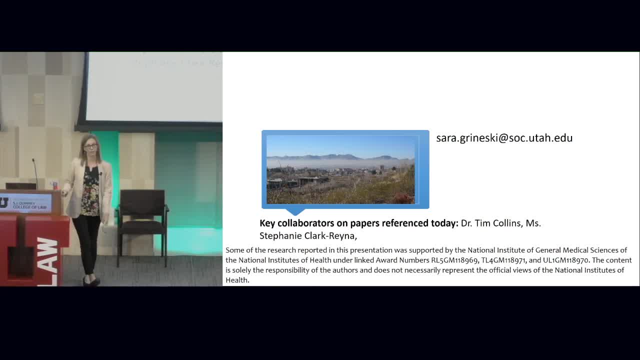 collaborators on the work are Dr Tim Collins. He's the co-director here at the Center for Natural and Technological Hazards with me- And then Stephanie Clark Raina, who's a former undergraduate and master's level RA at University of Texas, El Paso, and she's currently a doctoral candidate at 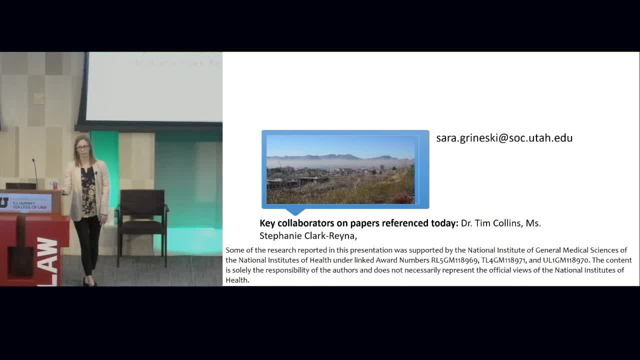 Northeastern University. So they were involved in all the research I presented today. So thank you. So I guess, if there are any questions, We do have time for some questions. We have microphones up here. Folks take advantage of this. 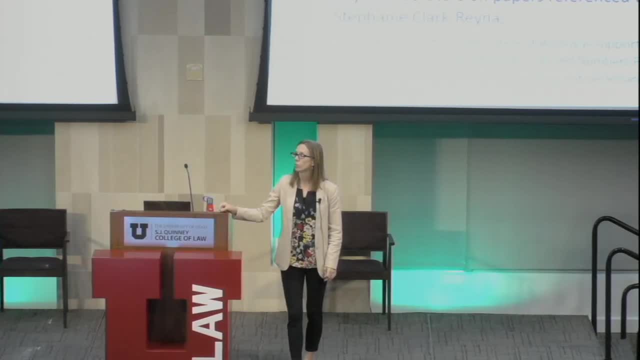 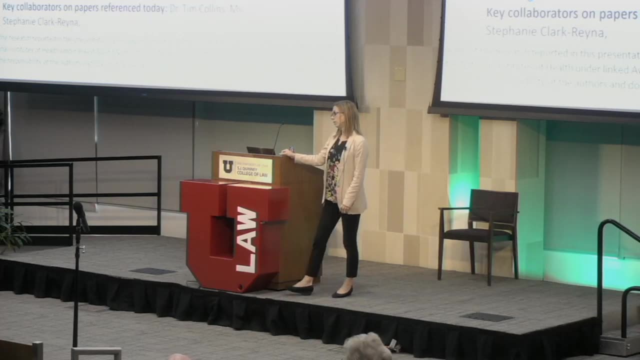 I'm curious about the effects of exercise which generally are thought to be good and helpful for the health of children. I'm curious about the effects of exercise which generally are thought to be good and helpful for the health of children, But in polluted environments, the deep breathing and all of that. what are the tradeoffs there? Do you have any insights there? 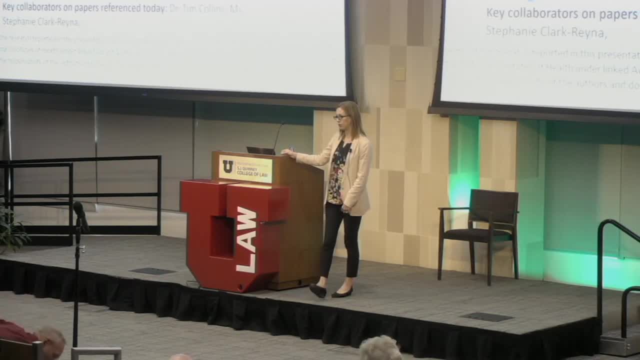 I do in a very limited way. I have read the literature that shows that exercise is good for executive function, And I've also read a study that I just came across last year that tried to answer this very question about when the air is bad. are you supposed to not exercise or should you still exercise? Because the benefits of exercise versus the benefits of taking in the air pollution And the study concluded that it was better to not stop exercising for long periods of time, That even if the air is bad, the benefits of exercising would outweigh the negatives of breathing in the air. 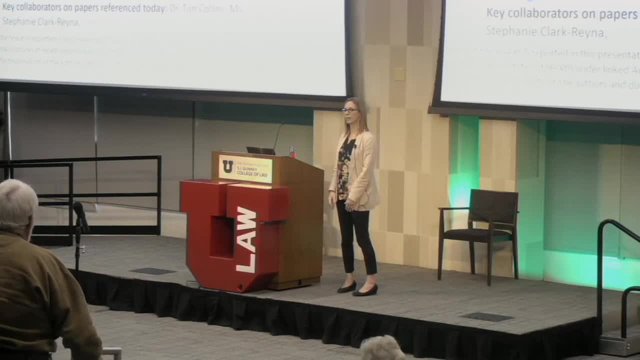 But I can't imagine that would be the case on like a red air day, Right. So I think if you were to continue to exercise because it is really good for you, but then make good decisions about when you exercise, Right, Using the local. 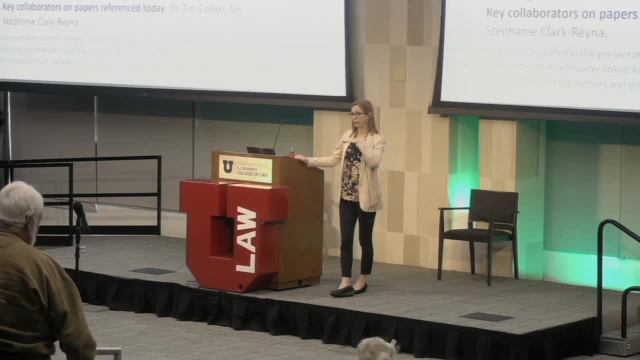 Air quality monitors like the AQ and you network of sensors that we have here. that's run by Carrie Kelly and her colleagues, where they actually have a map and people have air quality monitors of their house So you can find your house on the map. Like I know, there's a monitor a block from my house so I can see what the air quality is like at my house. 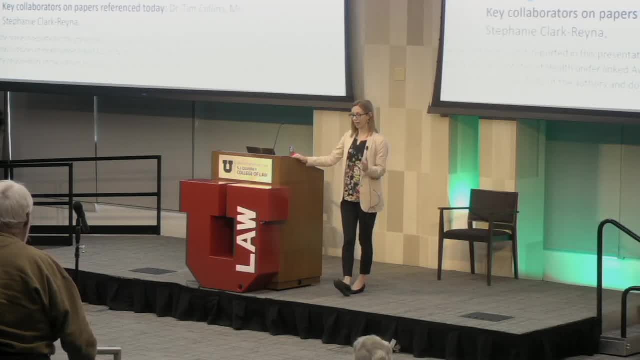 Right To try to make better decisions, But I don't think, based on what I read, the idea is not just to stop exercising, because there are a lot of benefits of that too, But certainly there are negatives of exercising while polluted. Yes, 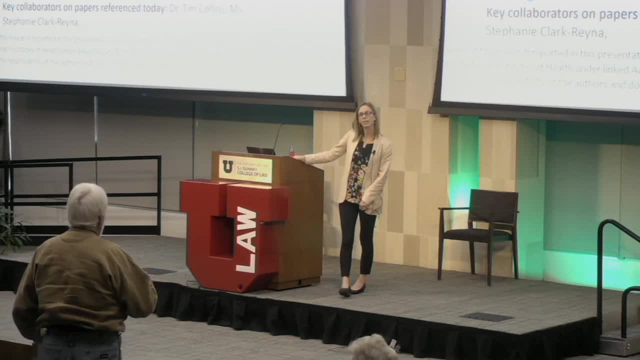 Hi Sarah, This is fantastic, Thank you. I'm wondering: you know this inland port project that we're fighting over and you know a certain amount of it? they've already. it's a done deal, Yes, But then you know they're trying to get them to at least do an environmental impact statement. 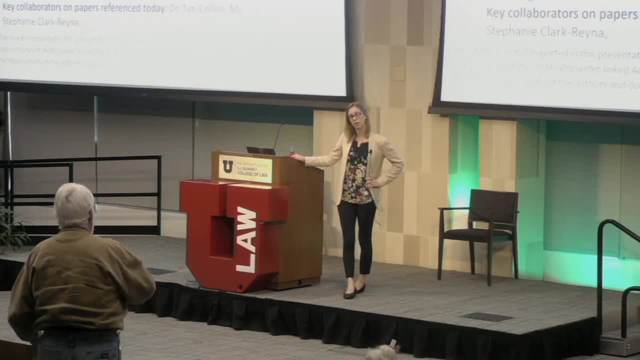 I wonder if there's anything that you guys are doing or you know as a group, to try and not. there's nothing we can do now to mitigate it, but we can at least study it and see how much the effect Is. 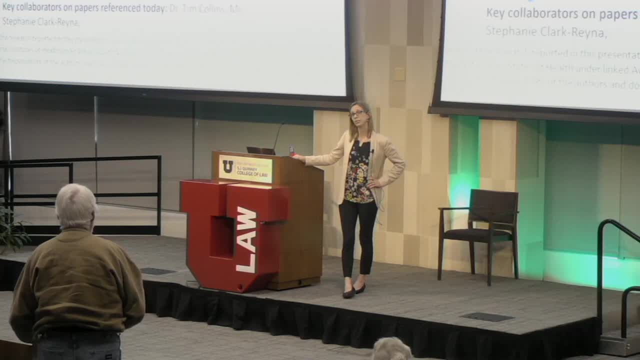 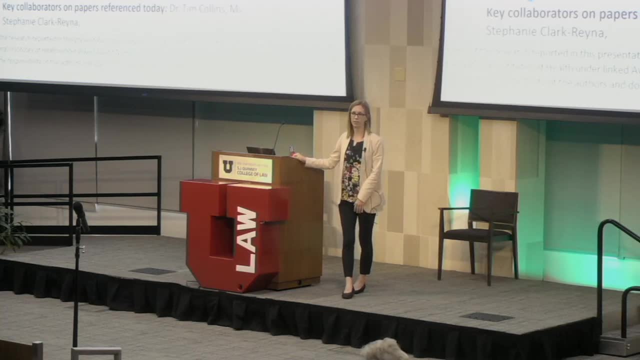 Yes, I don't know what your feelings are on that. Yeah, I think that's a great idea. I think it's something that the University of Utah, through either the Center for Natural and Technological Hazards or one of the other- you know many researchers on campus doing air quality related things. 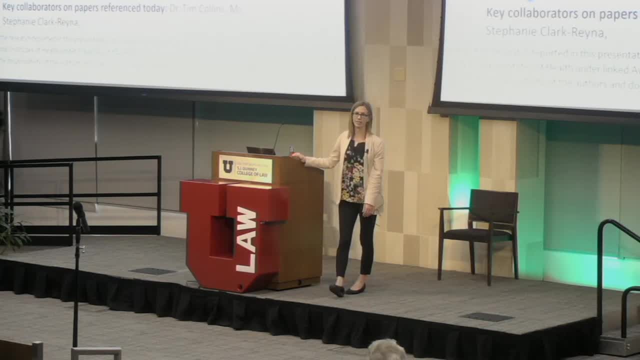 It does seem like being involved in the studies and then sort of continuing to do research on what are the consequences of the port, in hopes of providing information that's useful to decision makers in the future, would be a really, really good idea. So I work for an advocacy organization in Salt Lake that works on air quality: the Healthy Environment Alliance of Utah. 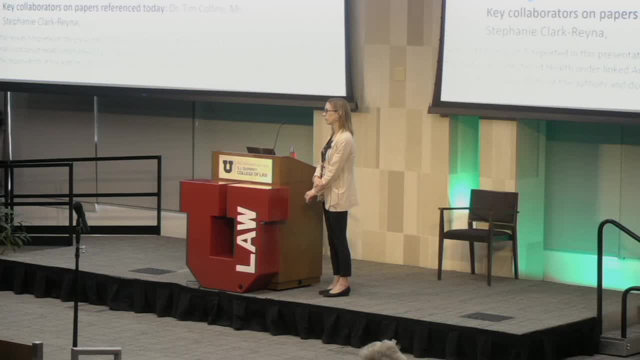 And I specifically work on our air quality campaign And not to totally put you on the spot, but kind of given all of this, like what would your like two or three like high level takeaways be for policy makers? 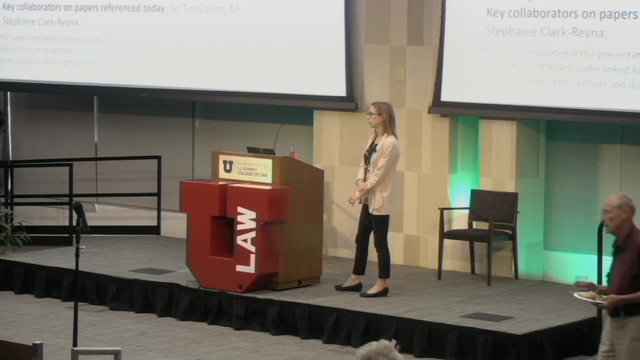 Because I think that air quality has increasingly become an issue that the legislature is paying attention to, which is awesome. Yeah, And you know, we've gotten a lot of funding. We've gotten a lot of funding for air quality in the last year or so, which is great. 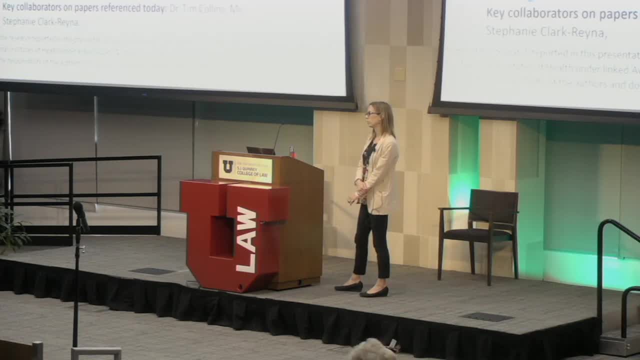 But how do we keep the conversation going to make them, you know, continue to think that this is an urgent problem and that just because we got $29 million last year, they're not going to forget about it this year? I see That's interesting. 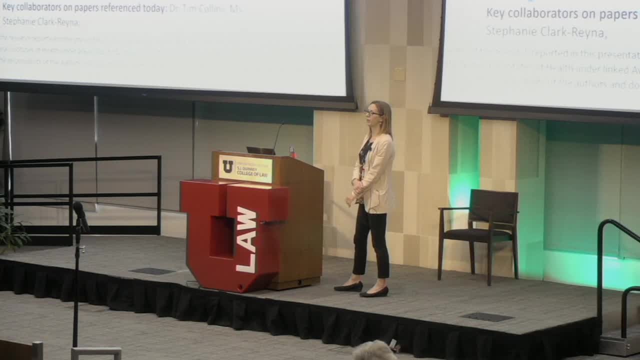 Yeah, I think I can only speak from my own experience, but I did like 10 years of research on asthma and environmental justice and air pollution And like it never seemed like I did a few little policy reports but it never really. 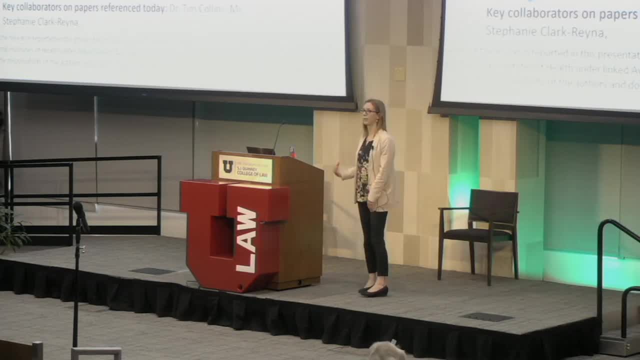 It never really caught anyone's attention. And then, when I started working on this topic of air pollution, environmental injustice and, you know, children's cognitive development, school performance- I don't know if the media environment has just changed, but it seems like this is something that's catching people's attention in a way that saying it makes it hard for kids to breathe isn't. And I don't know that it's better or worse. I mean, I've met many families that have horrendously challenging experiences- their children not being able to breathe- Like it's very serious, But I don't know if it just sort of became passe. 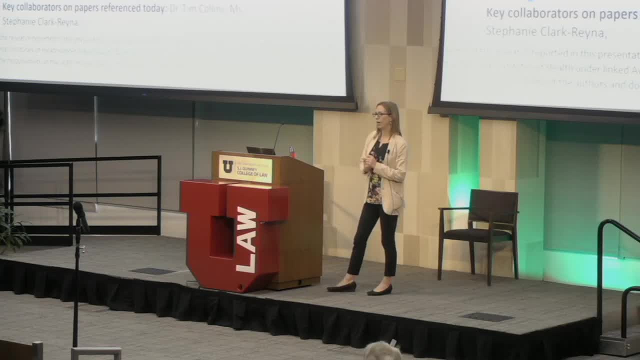 Like: oh, we all know that, you know. But I think that the focus on children's development and children's academic performance to me seems like a good hook for getting attention, Because we know that and I hate to use an economic logic because it's not motivating to me personally, but the logic that if kids aren't doing as well, then that might hurt the- I mean, they may not have as good of jobs. 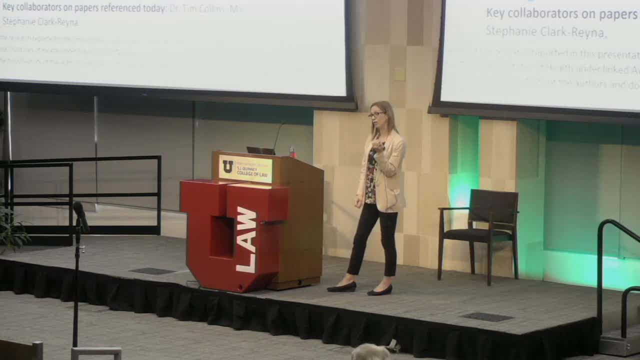 I mean that matters for them, but it also matters for our society as a whole. So if we think about decreases in human capital, Decreases in IQ, Decreases in scientific discovery Right, These things are all important at a societal level. 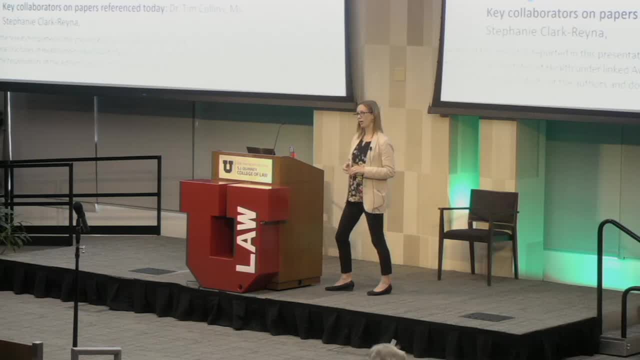 And so I don't know if framing it in that regard is helpful as a way to, you know, keep people's attention. And I also think the focus on kids helps. I mean, I consider, because I put a picture of my children on the slide, like it's a huge motivator of what you know, of what we care about. 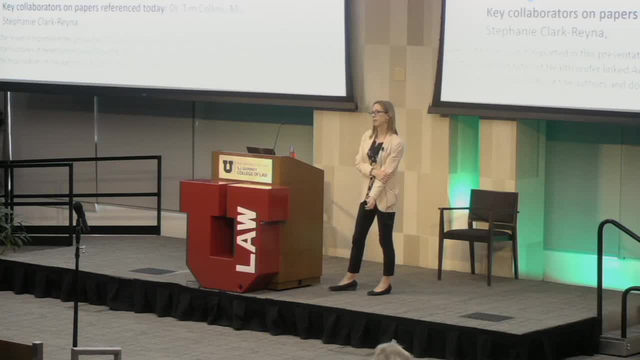 And I think especially in Utah. we care a lot about kids, And so I think the information about how children are being harmed and also that they're more harmed by the same level of pollutant than adults are- And there's a huge body of literature that supports that logic- 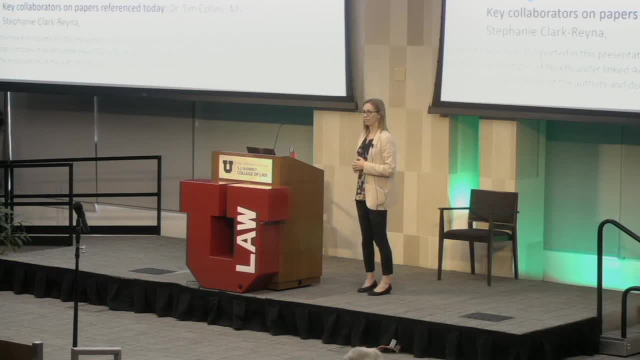 And so I also think that's another sort of framing technique. is that? I mean, we want the best for our children, I think as sort of a general narrative, Even though we don't always act in ways that make that happen. But I think it's something we think about. 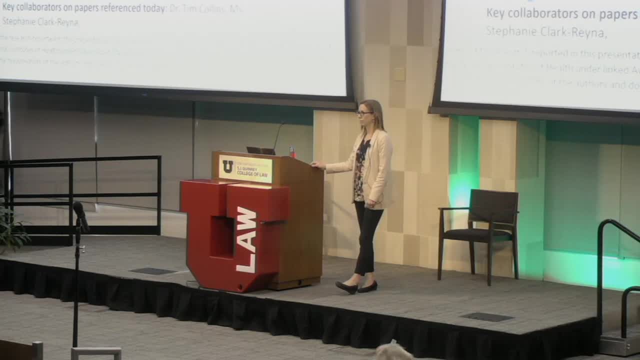 I don't know if that answers it. I actually had a question. I was intrigued by your data regarding school siting and the obvious effects on cognitive development of younger children. Is it more important to get the school siting right for elementary schools as opposed to the upper level schools? 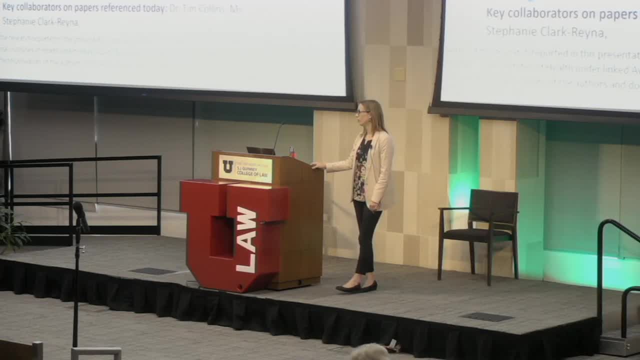 And is that more challenging because we have more elementary schools? Right, It's a site, Right? Yeah, we were interested in that finding And it took us a while to think about it And I was asked some questions about it in interviews about the study. 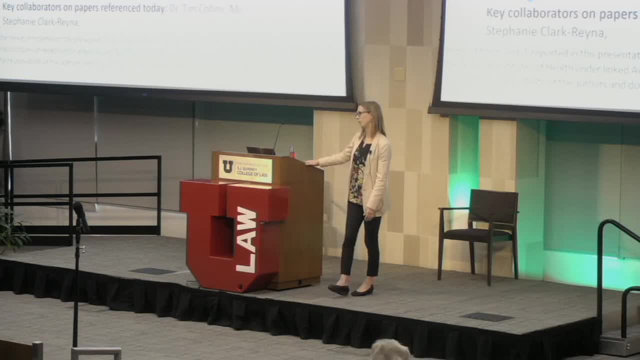 And it's sort of interesting that we have this disparity. and then how and why does it matter? But certainly the literature would suggest that critical windows of exposure would be more dangerous for younger children as compared to high school students. But if you're going to put someone in a polluted environment- which I don't want to put anyone in a polluted environment- right. 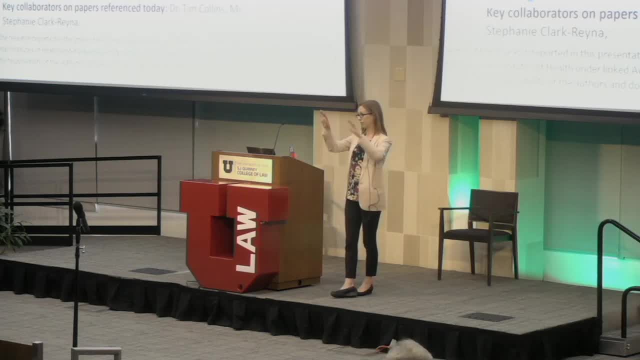 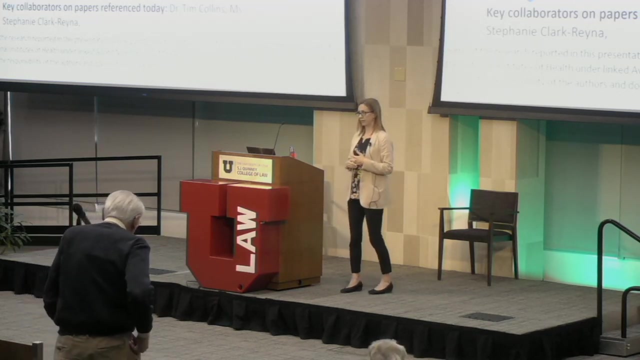 But putting the pre-K students in there is probably worse. It's worse at a societal level. Now, if it's your teenager, you don't want that student going to that polluted school yourself, right. But I think at a societal level, yeah, you would want to be the most protective of our youngest members because of their developing bodies. 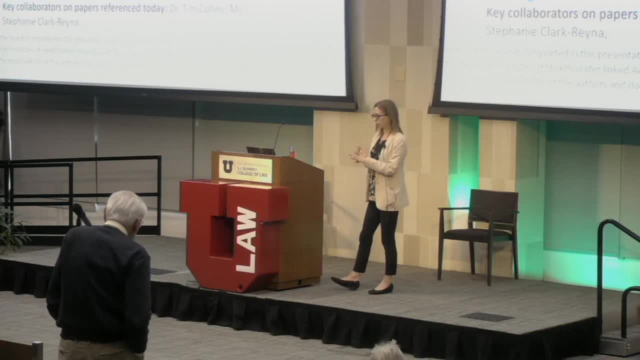 And I do think in part that the pre-K centers and the elementary schools. there are many more of them and they tend to be more of neighborhood schools versus like whole city wide high schools or regions of city, you know high schools, And so I think the 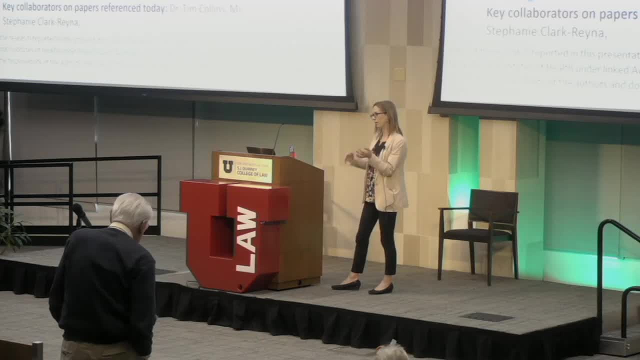 High schools are a little bit more dispersed, more likely to be located more in suburban or like less central city kind of areas at the national level than are the pre-K centers who you know. the Head Start centers go into low income neighborhoods and locate there where there is a great need. 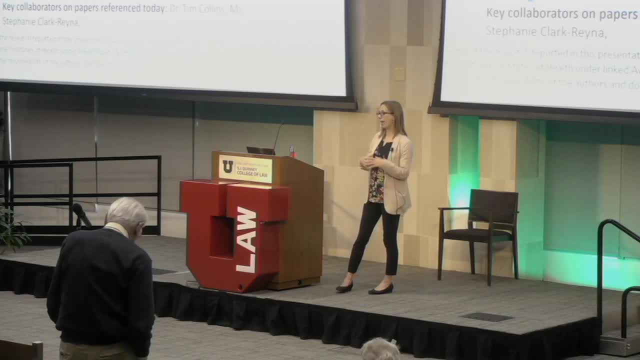 So I do think it's something about how we cite our schools, how we've organized our educational systems, But I do think it is concerning because younger children are more sensitive to the effects of exposure. We spend most of our time indoors, including the children in school, and indoor air pollution is much less than outdoor air pollution. 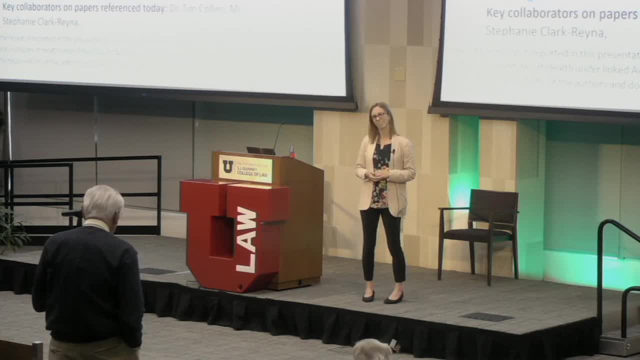 And so you almost need individual monitors, And there have been some studies where monitors are attached on school kids' backpacks and what have you? Has any of that, been that kind of data, been used for this, which is a little more accurate? Yes, it is much more. 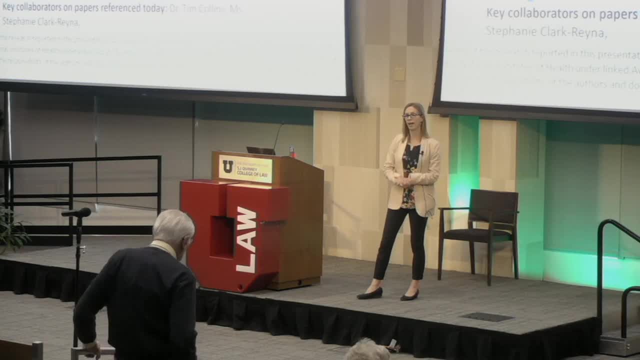 It is much more accurate in terms of generating, Generating actual exposure measures of people to measure something on their body. The newest technology are like little wristbands or little sensors that connect to their cell phones, So like the technology is off the charts now in terms of the ease of being able to collect that type of information from people. 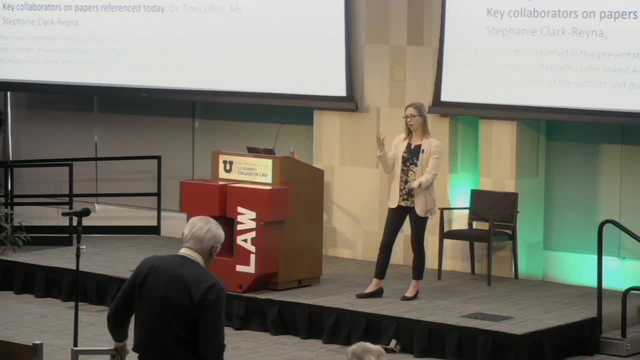 The trade off is that it's expensive, right? So you could do a small study with the wristbands, or I can use national level data right from all the schools in the United States and create this like sort of general national level Trend, And so I feel like if I could get like that data from every person in the United States, it would be amazing, right. 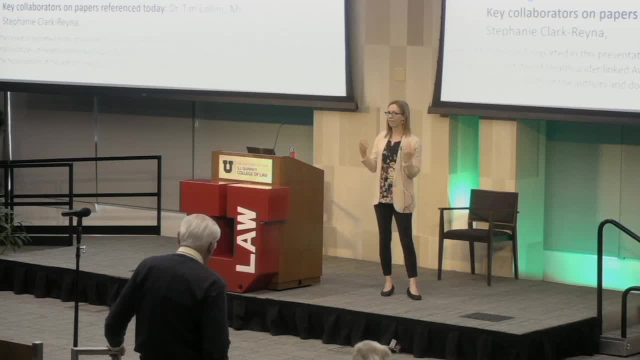 Or a large sample. But I think the trade off is, you know, the breadth versus the depth. So I think, the combination of both types of research, especially now, while the technology for measuring individual exposures is still pretty expensive, I can imagine a time, 10 or 20 years from now, where maybe it would be relatively- I don't want to say- easy. 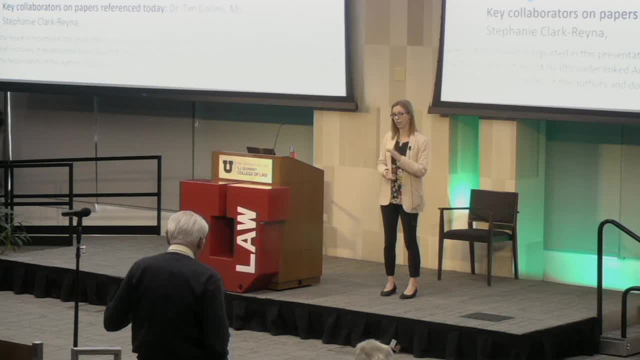 Nothing's easy right. It would be easier Right. And there is The AQ and U network here hosted by the University of Utah. they have some schools in the valley have monitors at the school and there's a team at Utah State and there's teams here at the University of Utah that are really interested in trying to get more air monitors into schools, outside the school as well, as you know, measuring the quality of air in the school. 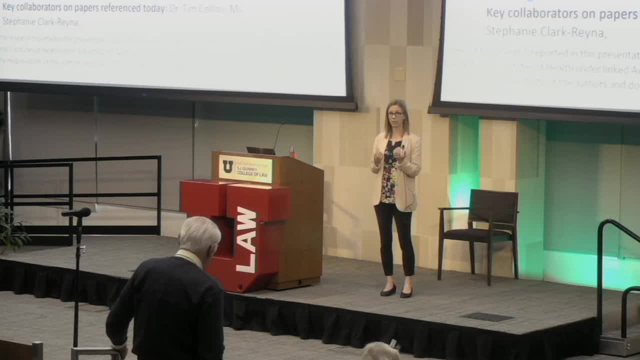 So, yes, it's definitely a direction the research is heading I'd be really interested in in that type of work on a more of a local scale, Because, you're right, We don't, we know. we do know that a fair amount of outdoor air gets inside and that outdoor air pollution is a key component of indoor air pollution. But there are many sources of indoor air pollution that are not captured at all, Like a mold, for example, that you might have from your- you know- leaky roof. cockroach allergen, which is very damaging to children's respiratory systems, particles from gas stoves. 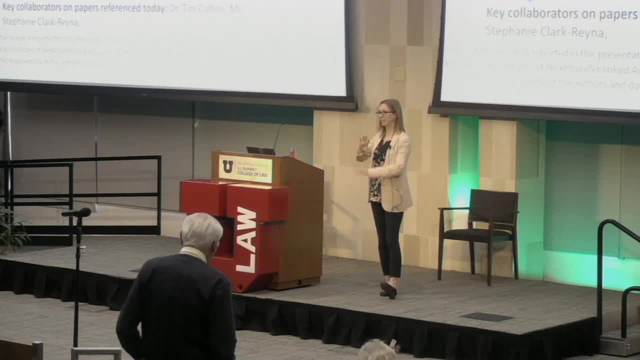 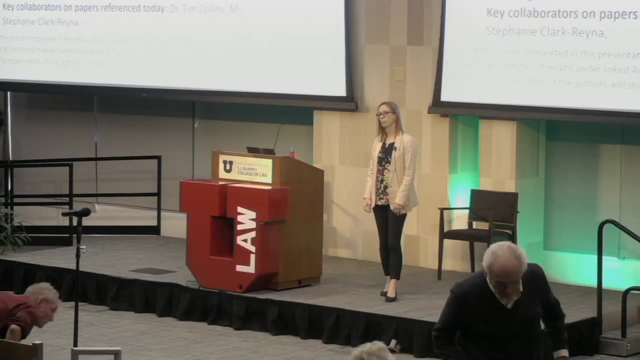 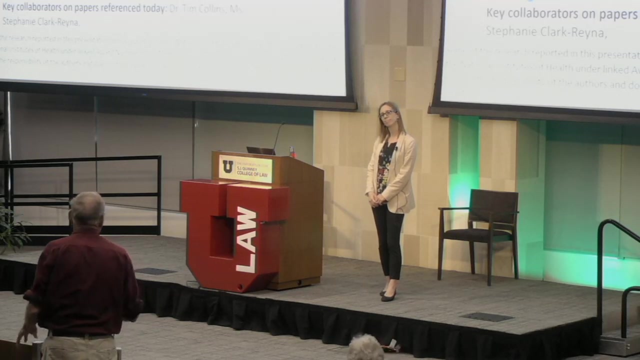 There's all kinds of sources of indoor pollution that what I've presented today is not at all captured in. Thank you, So for several over a decade- our nonprofit working with other nonprofits in this area of address this. I just want to make a point up a couple of things and then lead into a maybe some brainstorming. or the Utah Physicians for Clean Air. 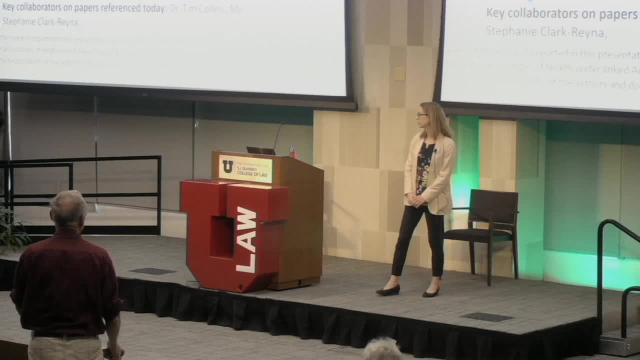 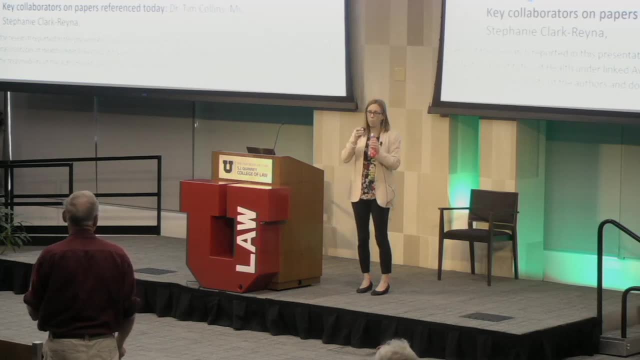 If you go to their website, they'll have a whole complete page On the neurological damages in brains of both adults and children, and their policy is to recommend any female who's going to contemplate pregnancy to leave the Wasatch Front due to the neurological damage that's going to occur in the fetus. 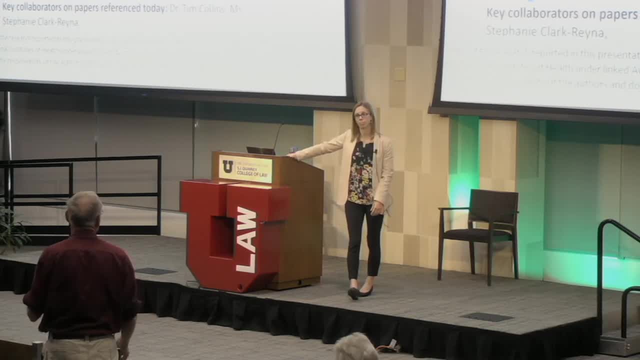 And we know Harvard and IH has done tracking on children in the United States over the couple of last decades. We have a three to five point IQ drop in the population, those younger people. They're not as smart as they used to be And that's correlated with that air pollution. 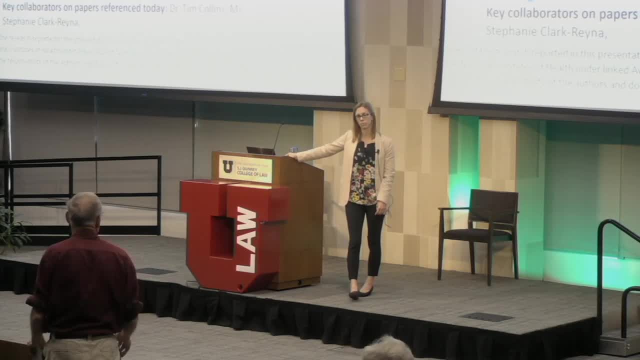 I know in my own home and the research we've done, you can put air filter systems in and if you walk into my home it's pristine And that air pollution. you're looking at singular schools, but the Wasatch Front. We mix that air all along from Santa Quint up the road up to Tremonton and, based on the Utah air quality studies, it's taking us all out. The cardiologist that does air pollution at the VA. there's 2,000 premature cardiovascular disease deaths every year, So it seems to me that there has to. we can do some things. There's a lot of different herbs and spices you can take beyond what you showed there. that'll hook onto those chemicals. 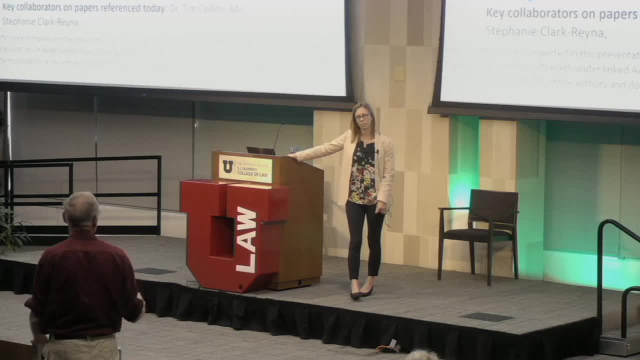 There's methods used by Russia, Japan and the US government in taking the body burden down, But it seems that we're going to be the only long-term. well, we can put those air filter systems into the school, but the only long-term solution, I believe, is going to be a political solution. 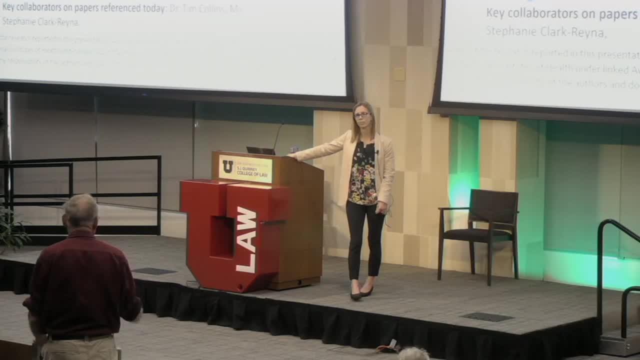 And that's when we get sick and tired of this. Have you guys addressed that? looked at that. It's great what you're doing, but until that reaches the governor's office and the legislature, I don't know that we're going to get a large movement in the air quality here. 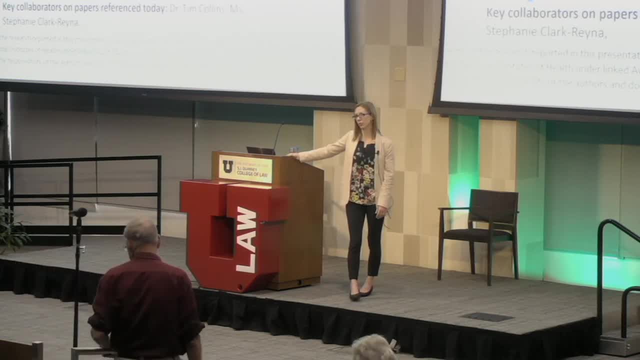 Right? No, I fully agree with you. That's why I was thinking. I mean we have to reduce the level of air pollution, right? I mean that's if we want to deal with these effects, Because we're finding even at, for example, with PM 2.5, at the tiniest of increase, we're seeing increased health effects. 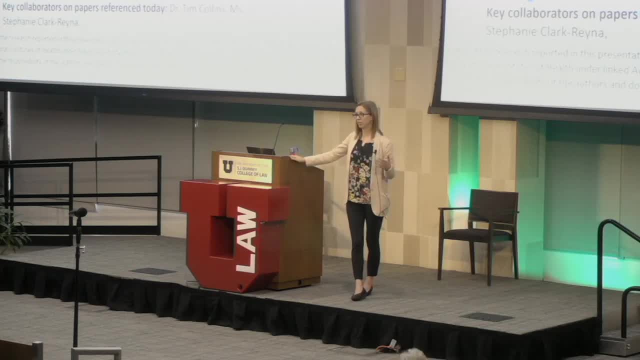 And so for a long time we thought the EPA still operates on this idea that there might be safe levels, but there really aren't safe levels of a lot of these things, And so I agree with you that a political solution, a regulatory solution, is absolutely essential. 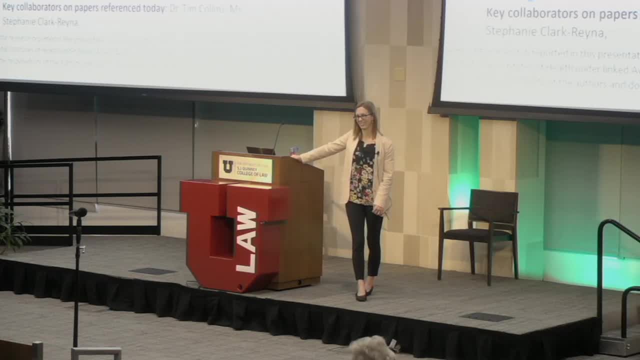 Now how to make that happen. I don't know Right. So before concluding today, let me remind folks that two weeks from today, the Stegner Center will host Professor Jason Robeson addressing Beyond Bears Ears: Post-Colonialism in Grand Canyon National Park, as part of our Young Scholars Series. 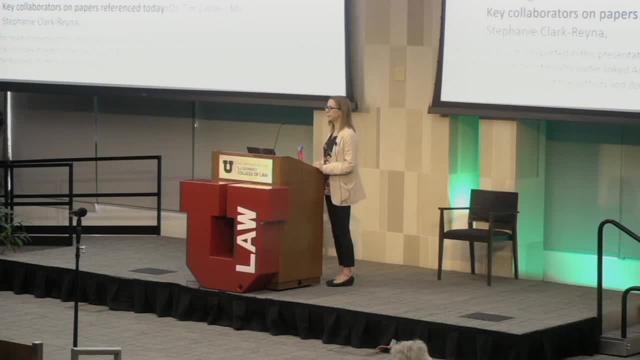 And with that let us thank Professor Grunewski. Thank you for a very timely talk.